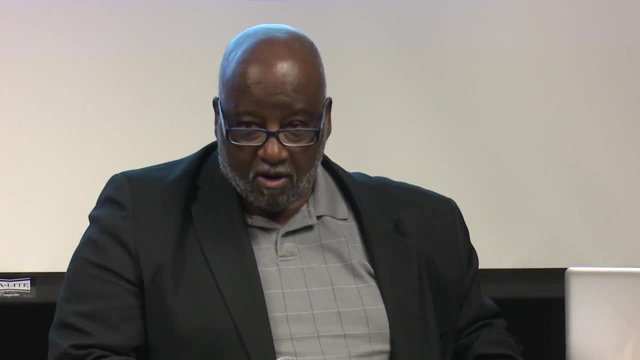 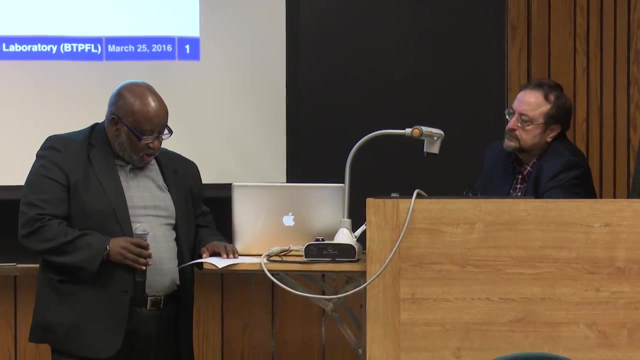 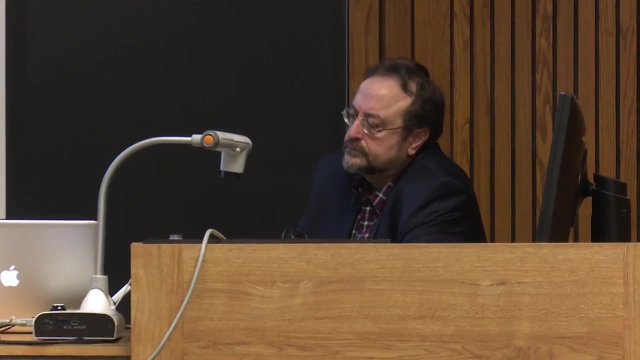 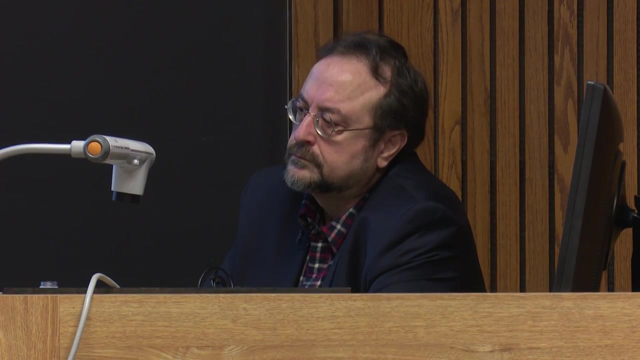 So now I'd like to briefly introduce today's speaker. It is professor Issam Mudawar. He joined Purdue University in 1984, and this was immediately after receiving his PhD in mechanical engineering, with a minor in management from MIT. At Purdue he founded the boiler, or the boiling and two-frame facility, the 120-to-water plant. 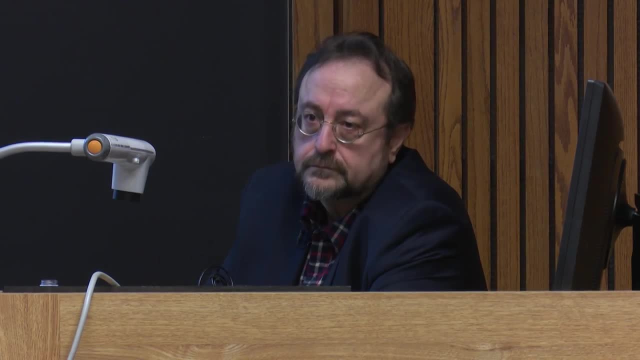 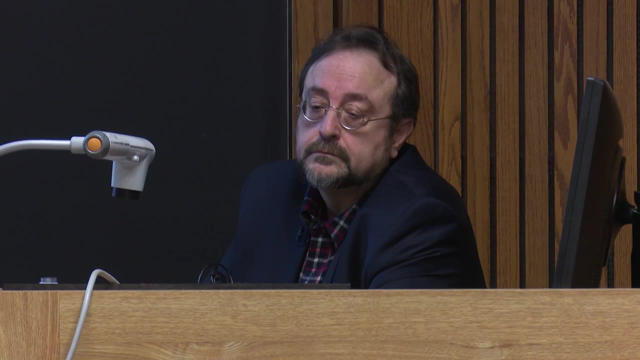 and the grigory was the base of the future of the college And the water a toboggan. and the water were used to ход the water two-phase flow laboratory, BTPFL, and the Purdue University International Electronic Cooling Alliance, the PUIECA. 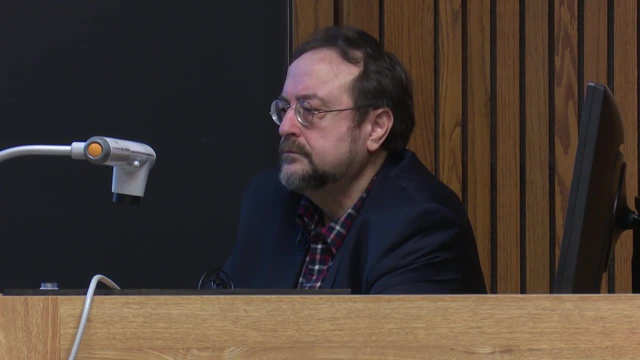 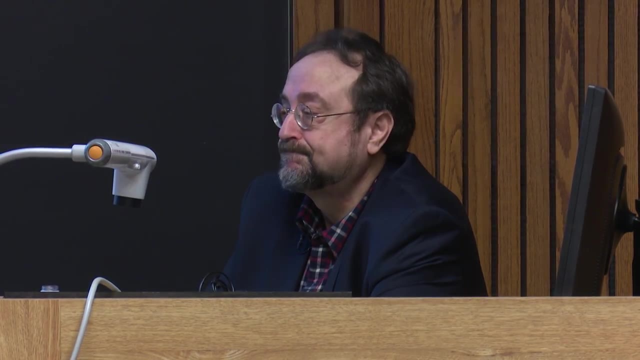 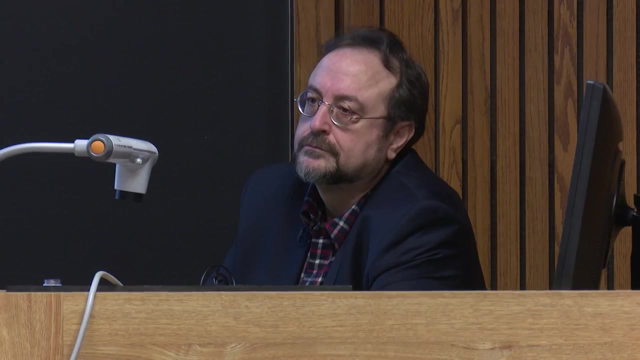 He is also founder and president of Moudoir Thermosystems Incorporated. He's a pretty busy person. This is a company that's based in the Purdue Research Park, And how many of you remember Paul Harvey? Do you remember Paul Harvey, the commentator? 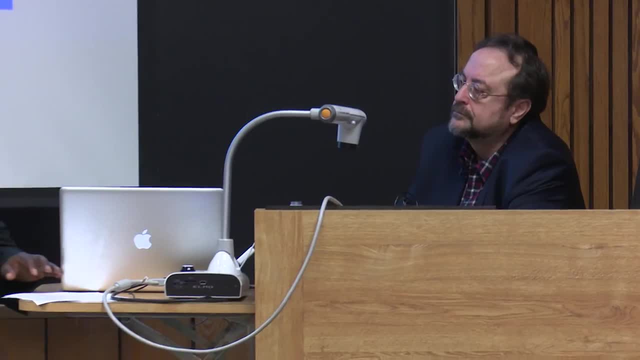 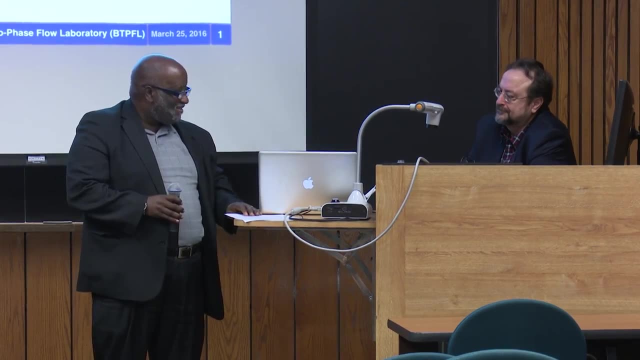 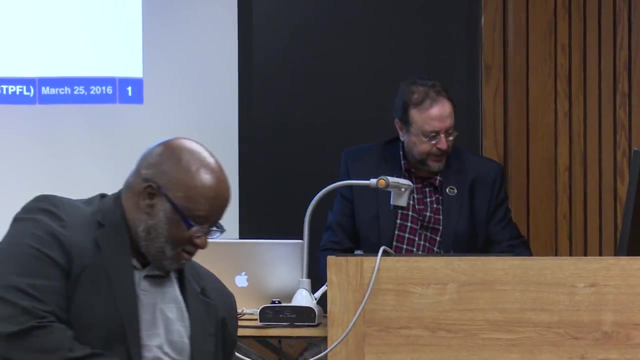 Following the expression, an expression from Paul Harvey. the rest of the story, I will ask Professor Moudoir to please share with us at this moment. Thank you, Thank you very much. All right, Thank you. I would like to thank everybody for joining us today. 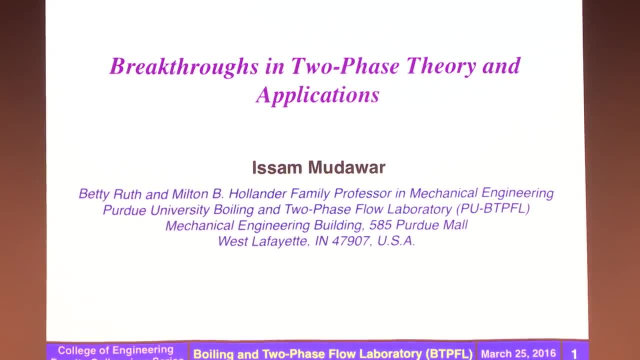 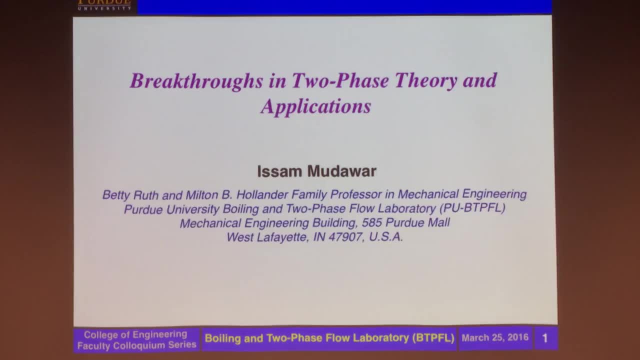 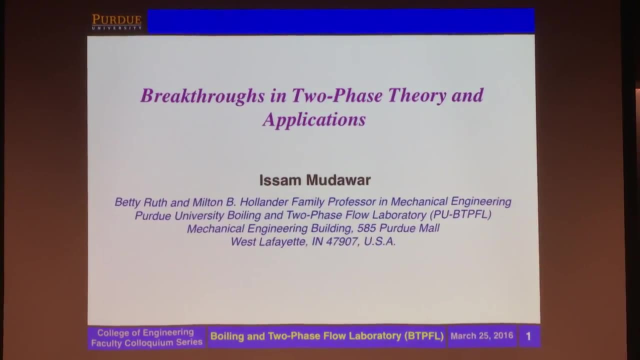 My goal with this presentation is to make it as informative as possible and, at the very end, just share some of my personal experiences about my 32 years here at Purdue, with some points of criticism, I guess, to the system that we have here. I think that's part of what we're doing with this colloquium. 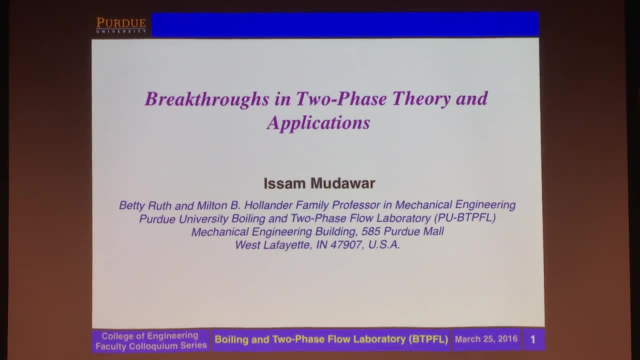 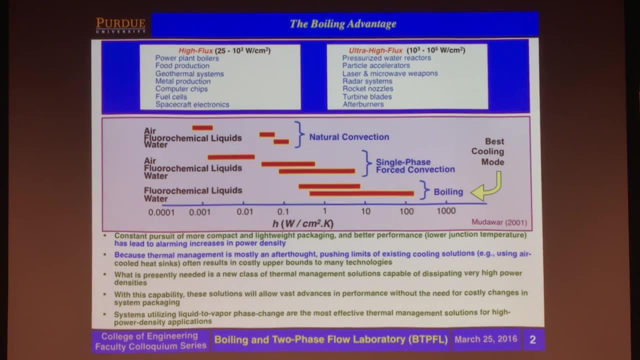 So I'm going to be talking about brainwashing. I'm going to be talking about the breakthroughs and two-phase theory and applications. I'm going to start that by looking at the different applications. where boiling heat transfer is very crucial today. You find that many of the advancements in all sorts of applications are becoming increasingly. 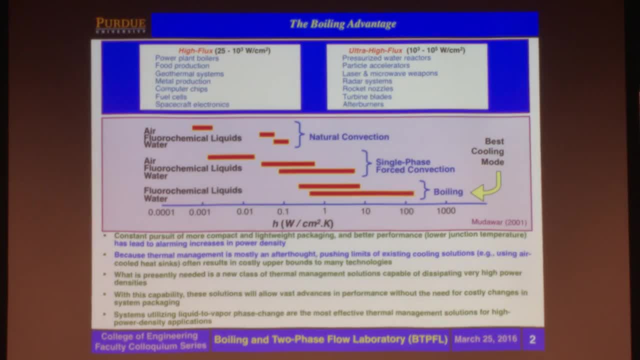 dependent on our ability to dissipate very large amount of heat from tiny little areas. Okay, So we're going to talk about the different applications. This is far away from the conventional mode of dissipating heat using standard heat exchangers and air cooling. 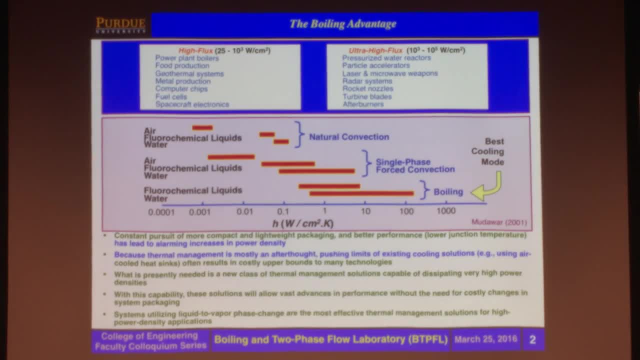 So, as a designer, you are given the opportunity to look at the different cooling modes that are possible- natural convection, using fans, for example, forced convection- And you quickly find out that boiling is, in many cases, the only mode available to really 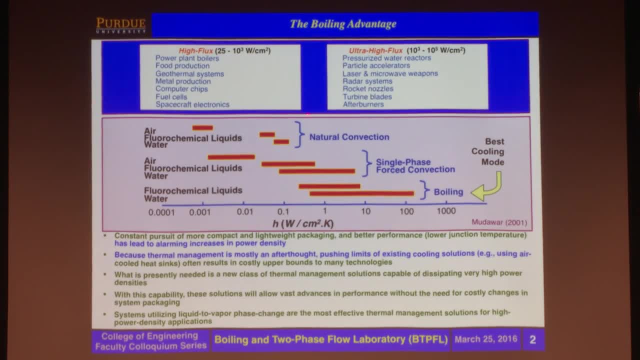 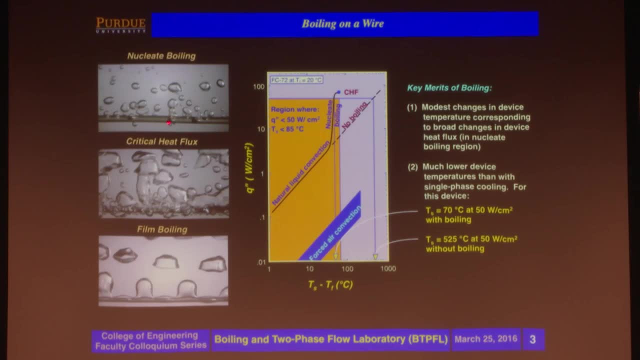 tackle the heat dissipation. Now, how does that work? I'm showing it here with a. this is actually a demo that I show in class. You're seeing boiling on a wire that is about a third of a millimeter in diameter. 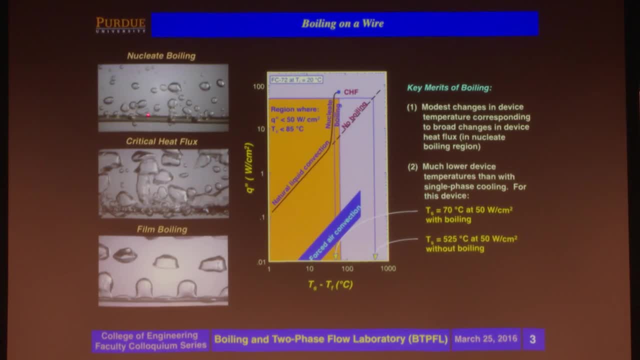 And this is really the mode that we're after: An abundance of bubbles formed at preferred nucleation sites along the surface, bubbles growing and quickly being removed by buoyancy or replaced by liquid at very high frequency, which is really responsible for a lot of the high heat fluxes that we get in this regime. 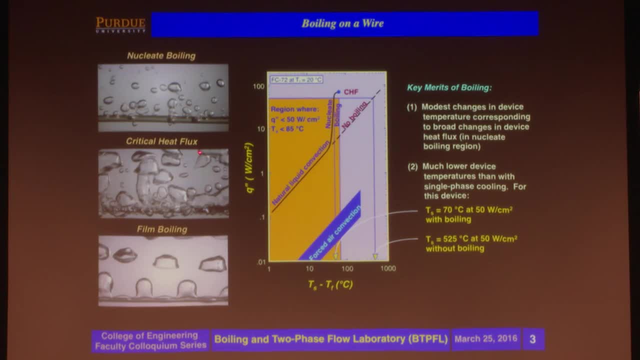 However, you have to be mindful of limitations, particularly critical heat flux- probably one of the most important parameters in these applications- where, if you overdo it with respect to the amount of vapor being produced, you suddenly blanket the entire surface with vapor, preventing liquid from coming back and replacing the vapor that has been produced. 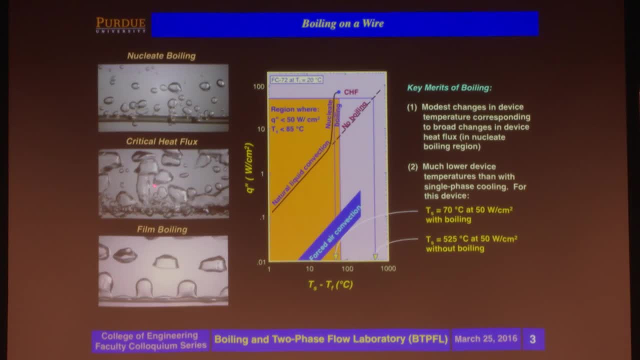 What is the net effect? It's a large increase in surface temperature. It's a very dangerous phenomenon, So you have to keep your operating conditions a certain percentage below this critical heat flux. Now in terms of the advantages of boiling, why boiling is so important. you can see them. 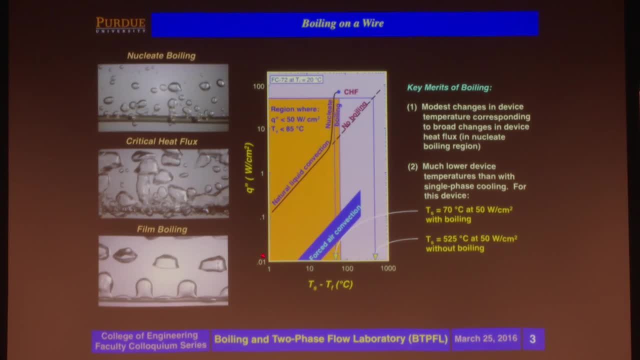 here with respect to a very simple application. This is an old device we had from IBM. We have a plot of heat flux versus temperature difference between the surface and the coolant, And the orange area that you see here is where you expect operation to take place. 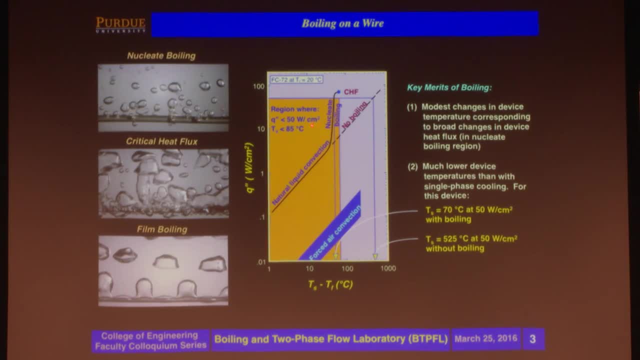 You want to dissipate heat fluxes up to 50 watts per square centimeter, but the device surface cannot exceed 85 degrees centigrade. And you could see, with forced air convection you're never going to be able to do it. 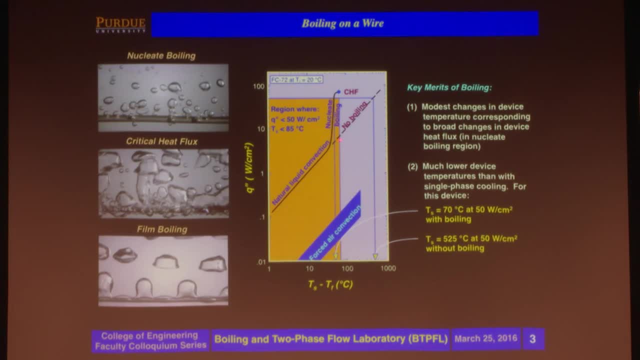 With natural liquid convection Without phase change. again, you find that by the time you hit the 50 watts you're going to reach 500 degrees. So if you are able to find a fluid with a boiling point say about 30 degrees below, 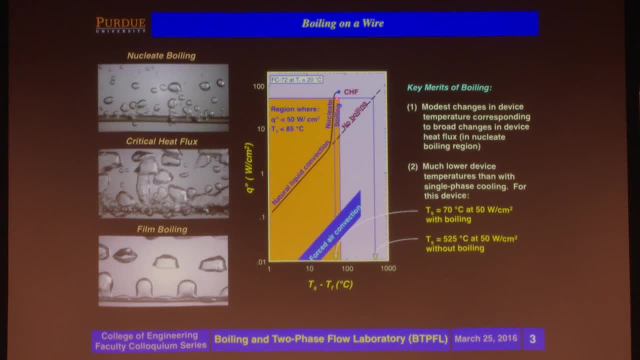 the maximum temperature. you see this large change in slope taking place right here, And what that does is allow you to maintain the surface temperature below 70 at the maximum flux, significantly less than the 525.. Not only that, there is another advantage, and that is the slope itself. 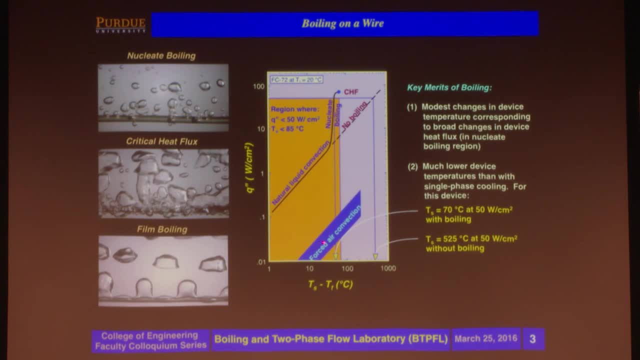 In many of these devices you have fluctuations in power and you're always concerned about the temperature changes that take place, because that's going to delaminate, cause cracking, cause stresses. So with boiling, what you're doing is allowing those fluctuations to take place. corresponding. 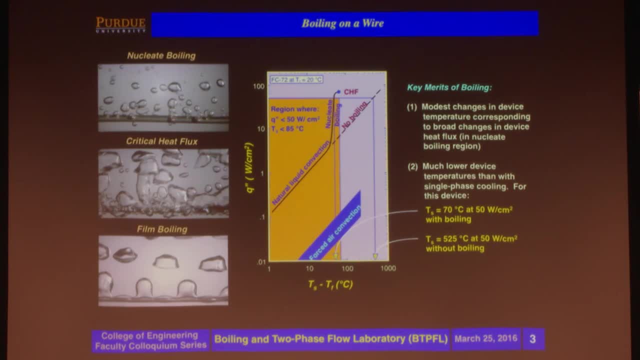 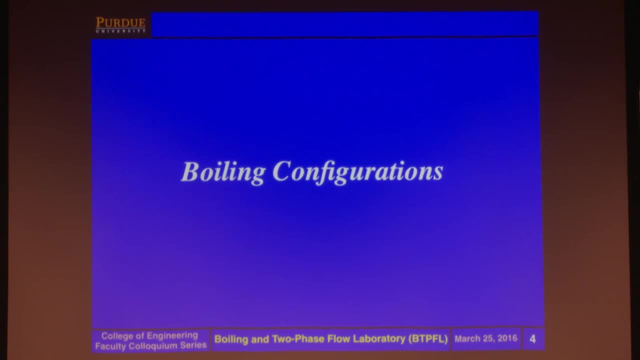 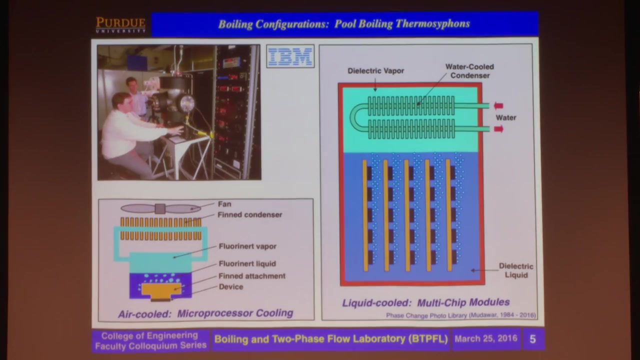 to very small changes in surface temperature. These are the two main advantages: 1. There is a lot of versatility when you look at the different boiling configurations. We were fortunate back in 1984 to have IBM and 3M support our experimental program related. 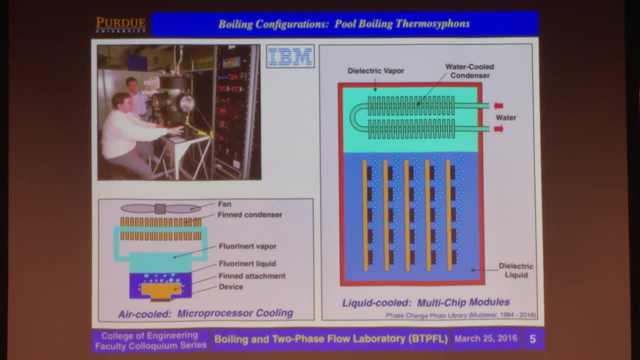 to high flux cooling. And, by the way, a lot of the facilities that you're going to see here are custom crafted by students. They're not purchased, So a lot of the work involved detailed design, detailed instrumentation. 2. We have a lot of technical equipment that we've developed over the years to be able 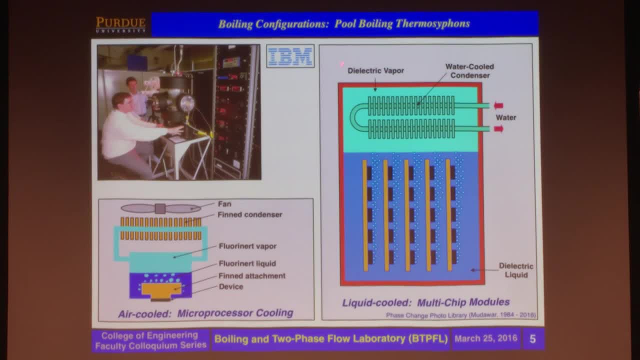 to bring it up to operational level. The simplest configuration is the thermal siphon that you see right here. At that time the thought was to submerge all the electronics of a mainframe in a pool of dielectric liquid. Heat is dissipated by forming bubbles which rise by buoyancy. 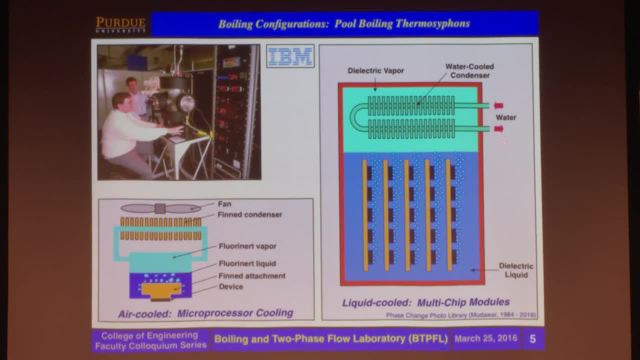 They are recondensed by a water-cooled condenser Within the system itself. there is no pump 3.. The thermal siphon is relatively driven and that's a major advantage, obviously from a cost and reliability standpoint. 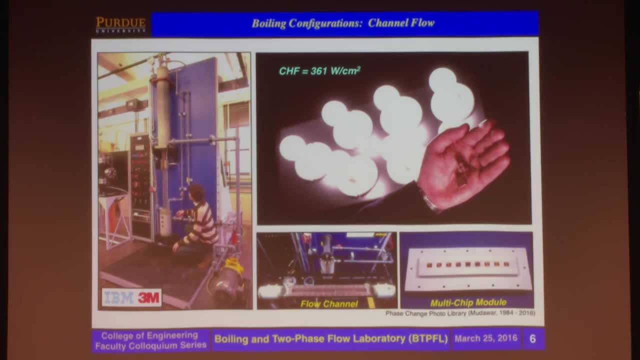 Now, when thermal siphons don't work, you start utilizing convection as a mode to enhance heat transfer. and what you're doing here is supplying the fluid at a certain velocity, parallel to the device surface, to take advantage of motion, And the higher the velocity, the better the heat transfer, obviously. 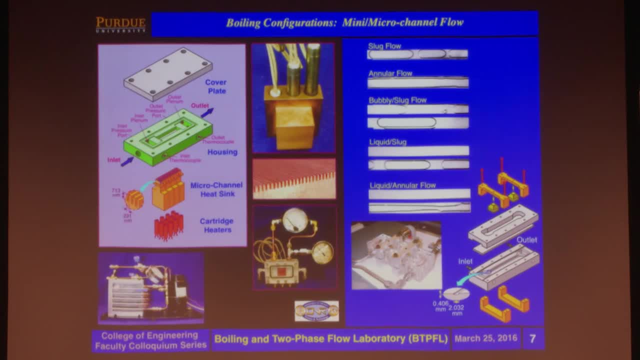 4. And one special case of forced convection boiling is mini and microchannels. They're extremely popular right now in many, many industries. What they do is allow you to reduce the amount of coolant that is required, greatly increase the heat transfer coefficient, but they have their own limitations as well. 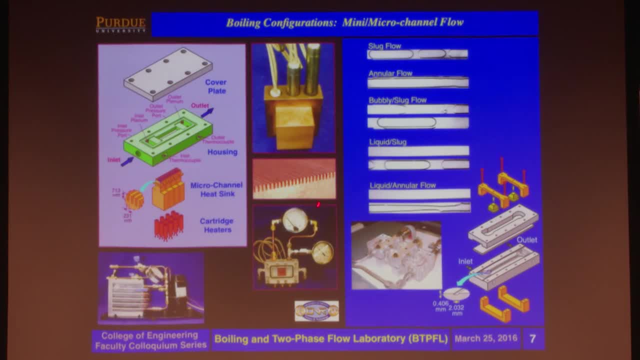 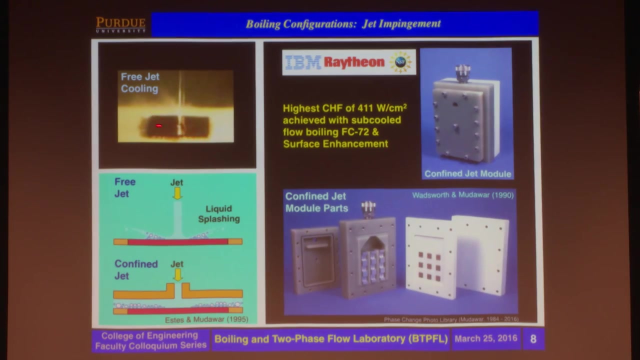 I'm going to talk about that later on. We're talking here about for mini channels about 2 millimeters- 5. Microchannels typically anything less than half a millimeter in hydraulic diameter, And when that doesn't work effectively you resort to jet impingement cooling where you 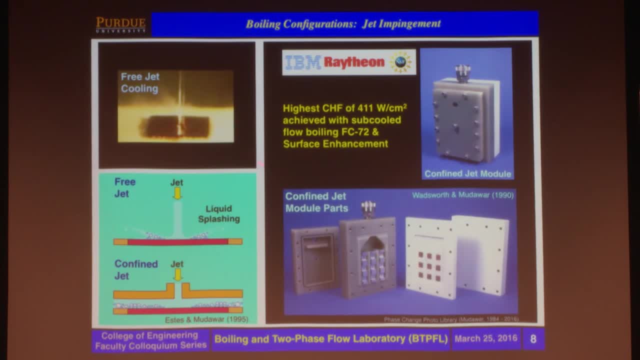 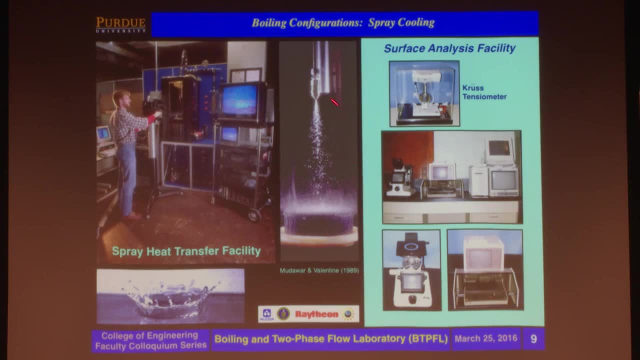 are bombarding the surface with a liquid jet And again, the higher the velocity, the better heat transfer. you get A competitor to spray cooling, to jet impingement cooling is spray cooling, which is what you see here. What you're doing differently is breaking the liquid into tiny little droplets before. 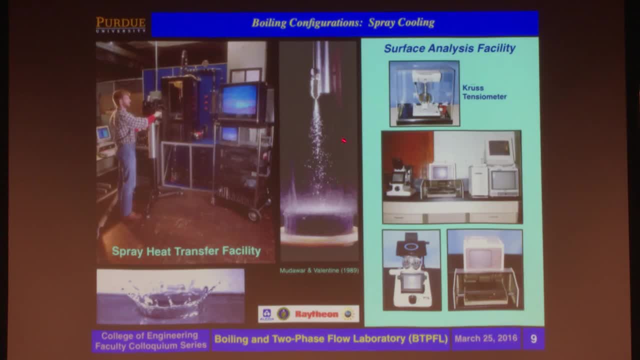 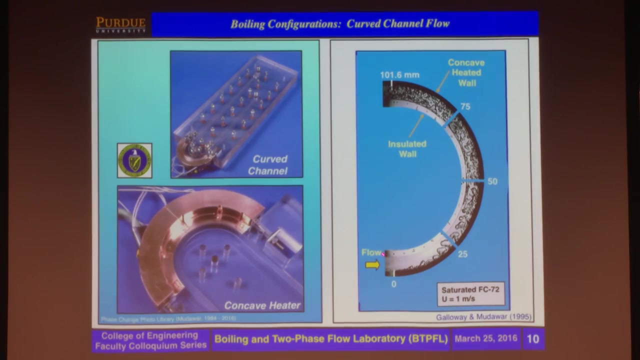 they hit the surface And what you're doing effectively is increasing the surface area to volume ratio of droplets, which is very advantageous for heat transfer. There are also specialized configurations for boiling, such as boiling in curved channels. Also, you can take advantage of curvature. 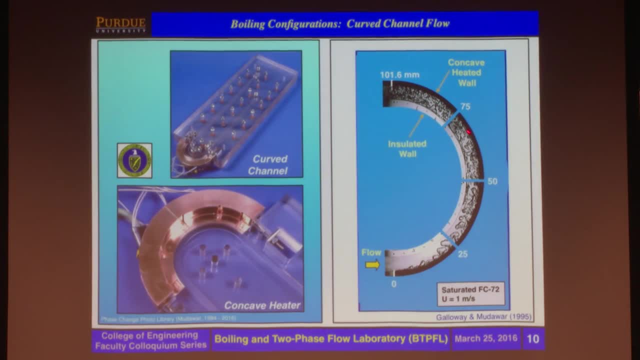 Here you have a heated concave wall And what you're doing is supplying the liquid with curvature, producing a centrifugal force, which we'll talk about in a minute would pull vapor inward and push liquid outward, which is exactly what you need to do. 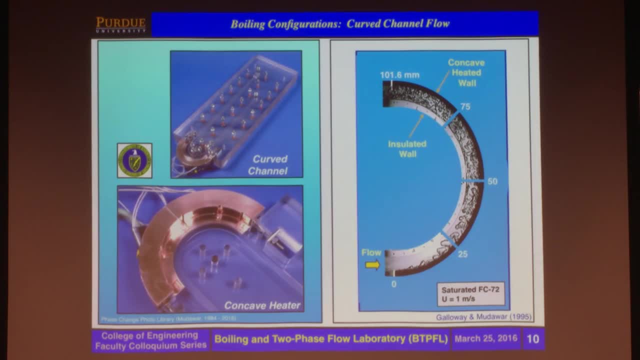 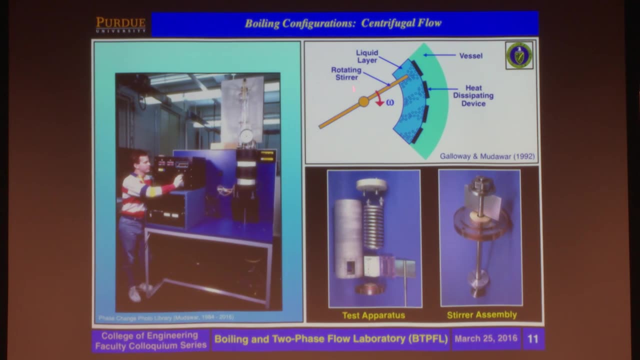 And with the higher centrifugal force you get even better performance. Or you can do the same thing with rotation, by spinning liquid at a certain rotational speed and achieving the same centrifugal effect. And what is nice about this is, again, there is no limit to how far you can enhance your 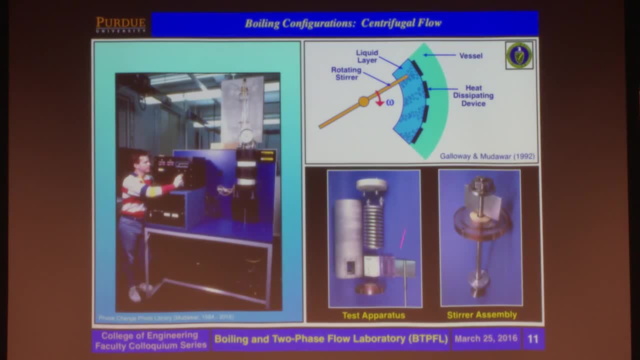 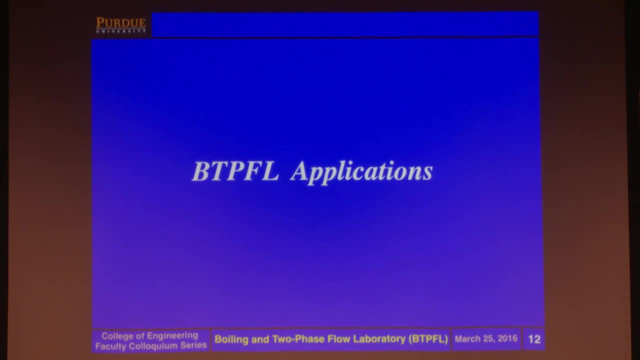 heat transfer If you rotate at 600 degrees, If you rotate at 600 RPM versus 100, you're going to get much, much better heat transfer. So all of these were tested in our lab as means to enhance boiling heat transfer. 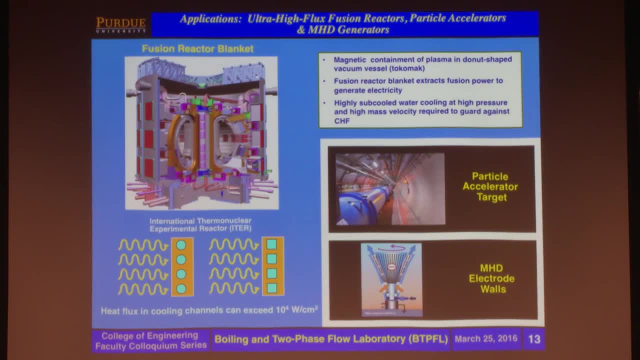 Now, in terms of the specific applications, I'm just going to quickly go through those. We have looked into several applications we call the ultra-high flux applications, And here we're talking about 10,000 watts per square centimeters and above The typically. 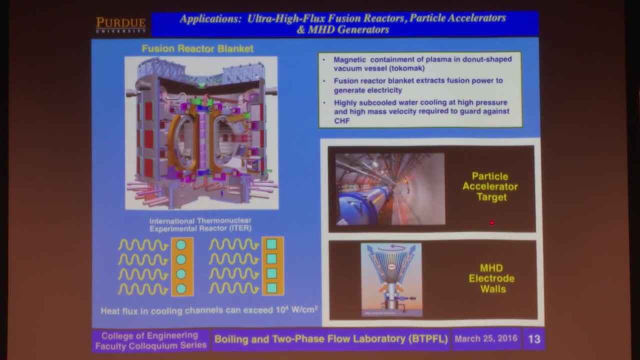 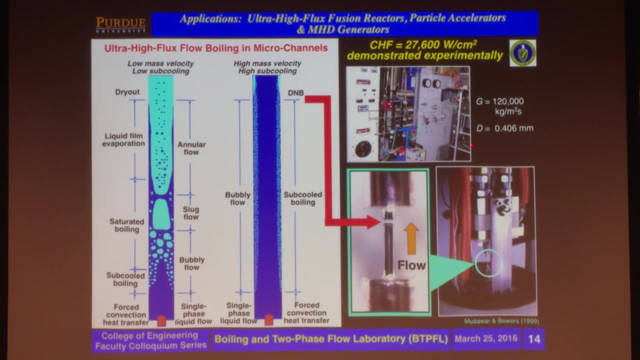 We typically encounter infusion reactors, particle accelerators, MHD electrode walls, And we have developed a special high-pressure facility here for this purpose. It takes us up to the critical point for water And at the heart of the facility is the apparatus you see right here where you supply 700 amps. 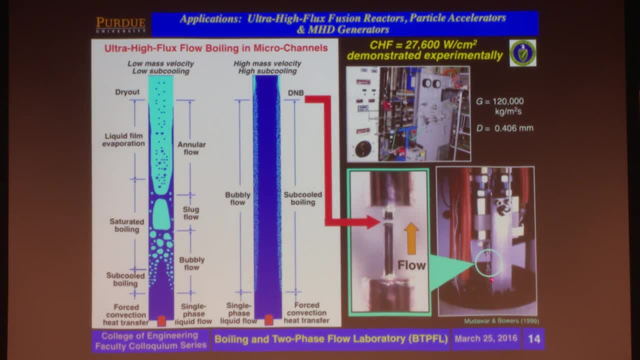 up to 700 amps through a tiny little tube. That's where the flow is taking place And you crank up the power until the tube burns. You get the critical heat flux phenomenon I talked about earlier, And this gave us a record- still a record- for critical heat flux in tubes: 27,000 watts. per square centimeter. That's 270 light bulbs, by the way, if you want to get a feel for that Dissipating heat out of an area half the size of a postage stamp- Another area we have worked on, particularly in the 90s. 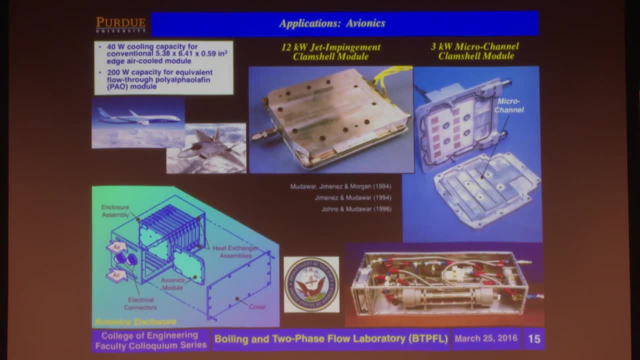 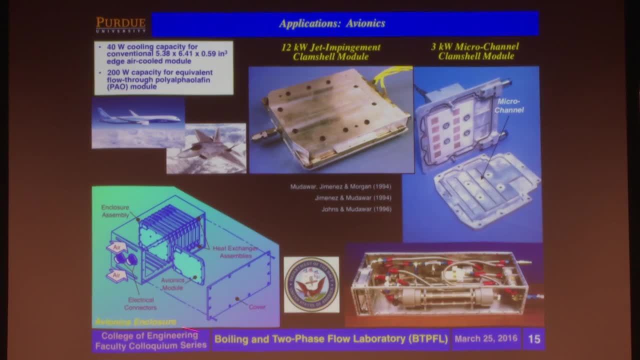 I'm sorry, Dissipating heat out of a postage stamp And, of course, one of these was avionics. This is the electronics for both commercial and military aircraft And in most applications, what you're doing is cooling the electronic using the avionics. 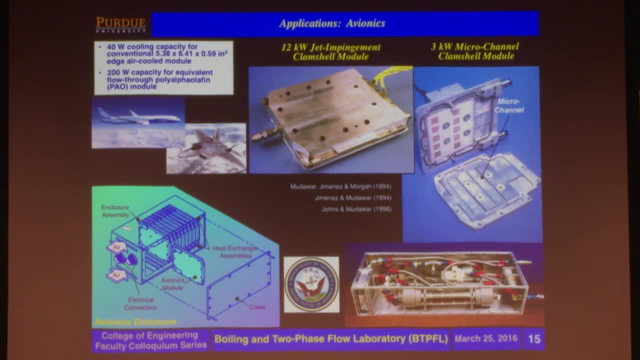 enclosure or avionics box. It's a rectangular box like what you see here, And the circuit ports are slid into it And air is used to cool it. Now, these modules- typically they are standardized. They're about this size. 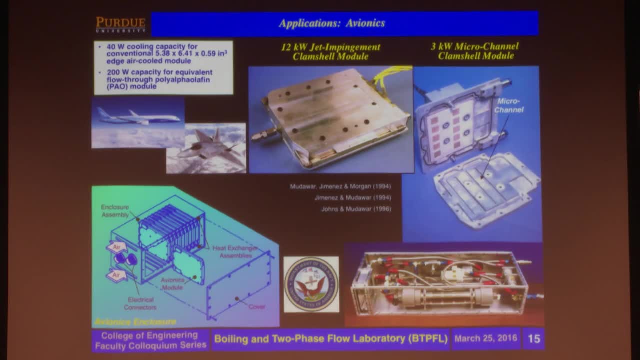 You can put it in the palm of your hand Back to theード, And they dissipate only about 40 watts because of a lot of limitations in terms of flow rates and pressure drops, whatever. Now, with phase change, we quickly changed that. 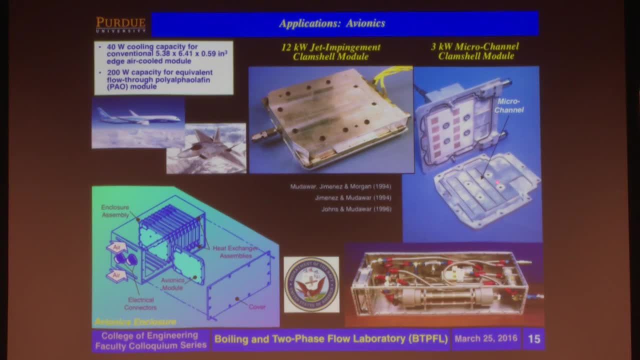 We did work in the 90s where we used microchannels and were able to boost that to 3 kilowatts And then with jet impingement to 12 kilowatts. And there are a lot of intricate features. There is a lot of design work, more than heat transfer work. 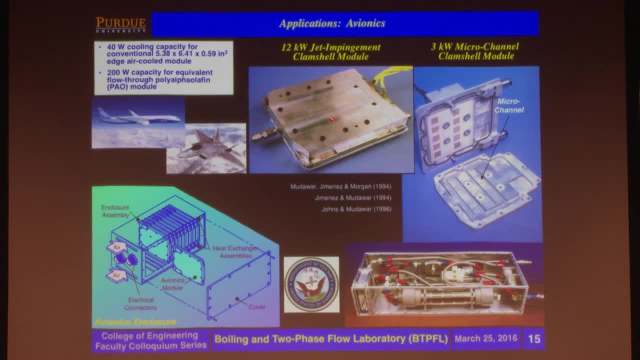 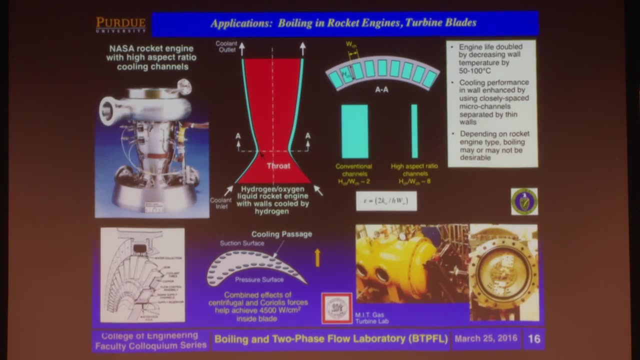 within these modules And you're talking about orders of magnitude enhancement just by means of utilizing phase change. We also looked at curve channels in conjunction with rocket nozzles. We looked at turbine blade cooling also, And at Zucrow Lab we did recent work. 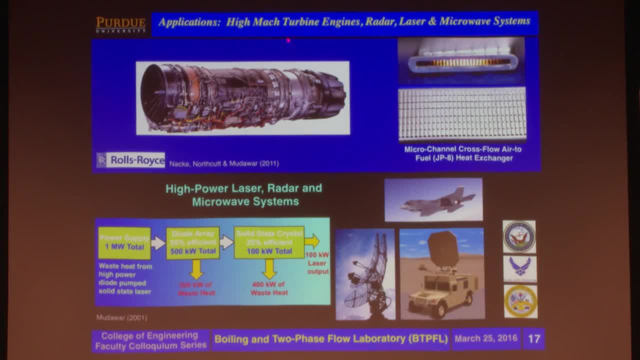 related to high Mach turbine engines. This is where you have compressors producing air at such a high temperature that they are no longer providing air that can be used for cooling in downstream parts of the engine, So the cooling air has to be cooled itself. 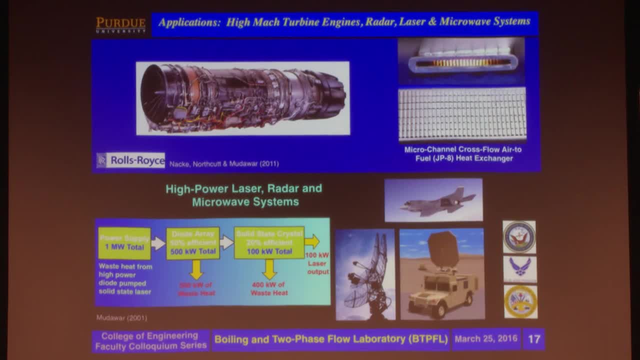 And the way you do it is by using specialized heat exchangers that suck the heat out of the compressor air and send it to the fuel, the cold fuel that is available on the aircraft, And we developed a cooling module that you see right here. 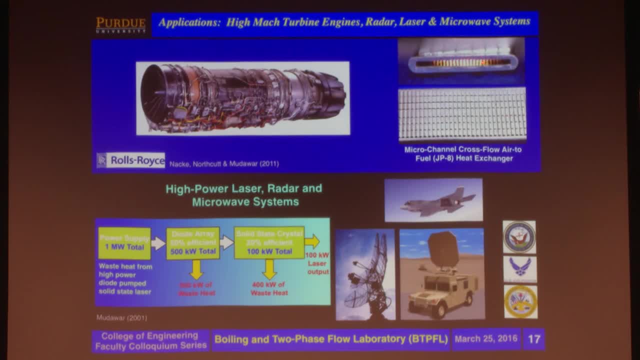 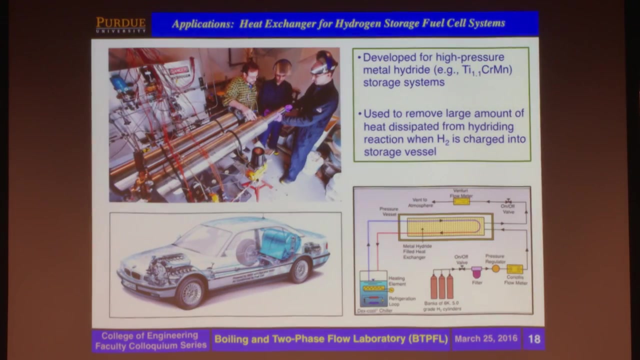 very compact cooling module where the fuel passes through the inside and air on the outside in cross flow And you can package those modules in whatever configuration you want to get a three-dimensional heat exchanger package. We also did a lot of work related to high power lasers. 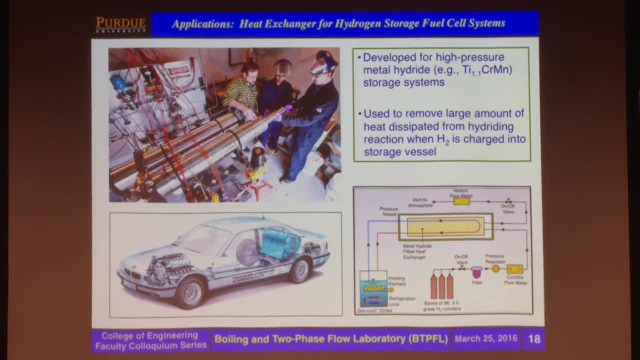 radar microwave systems using phase change as well. At Zucrow we also did work related to hydrogen storage fuel cell systems. Here we're talking about storing hydrogen in high pressure metal hydride. You supply the hydrogen and store it by reaction with the high pressure metal hydride. 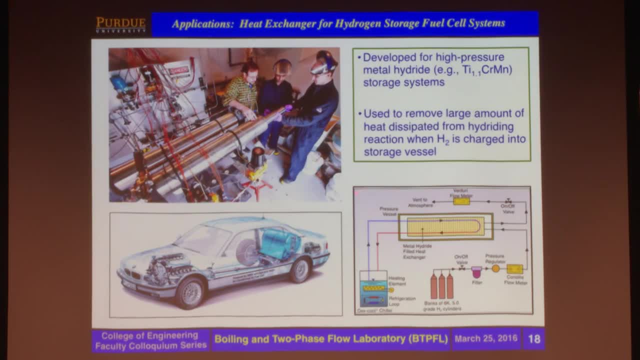 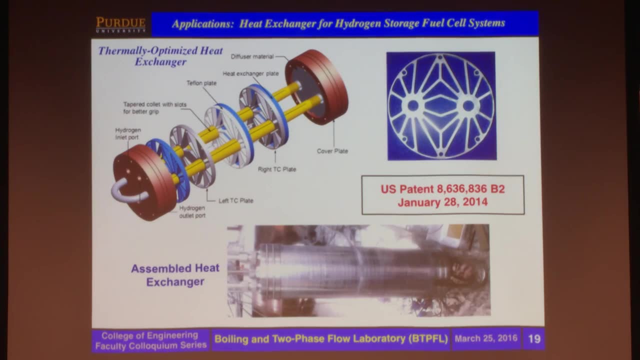 The problem with this is that you produce enormous amount of heat over a very short period of time, And we developed three different heat exchanger designs for this purpose, highly optimized thermally, And here you have one of them. You could see the shape where the heat is optimized. 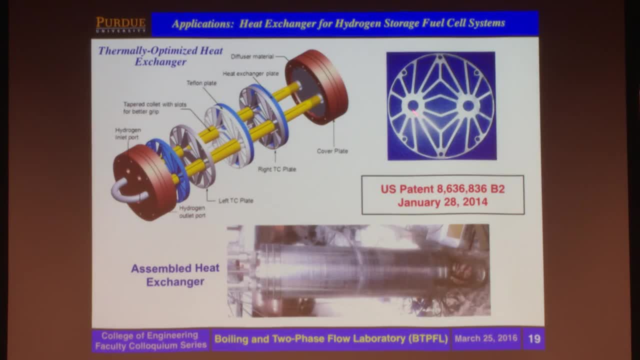 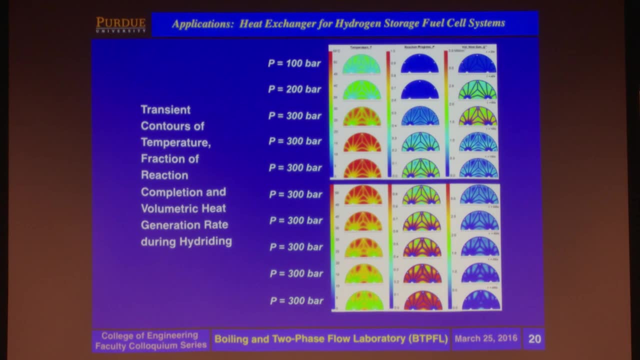 so that you fill the cavity with the hydride. And these are the cooling ports on the inside. And, by the way, these are very unique types of heat exchanger because they are transient heat exchanger, They are operating over a few minutes. 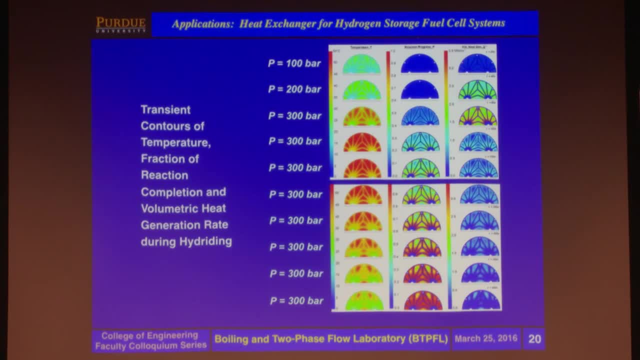 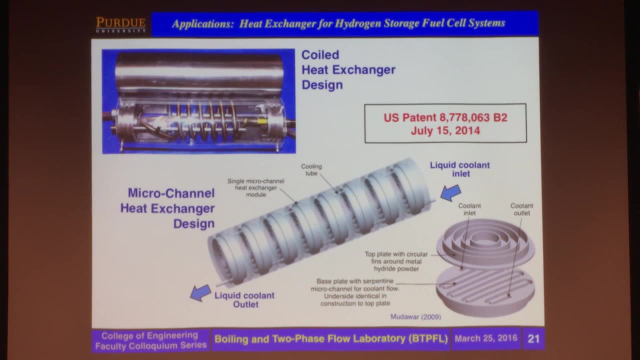 That's it. That's where you get this enormous heat dissipation. It's very different from conventional heat exchanger working on a steady state basis, And these are two different designs. other designs: a coil-type heat exchanger and these disk-shaped microchannel. 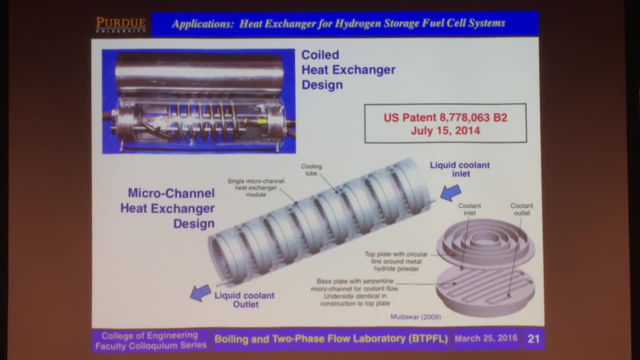 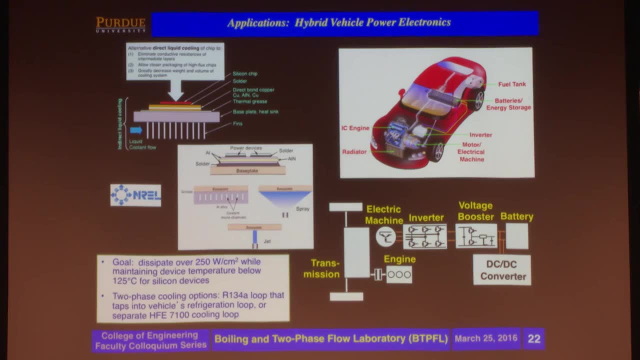 heat exchangers are stacked to store the hydride. Another area of interest has been hybrid vehicle power electronics. This is work we did actually at my company, not at Purdue was NREL in Colorado And again the idea is to 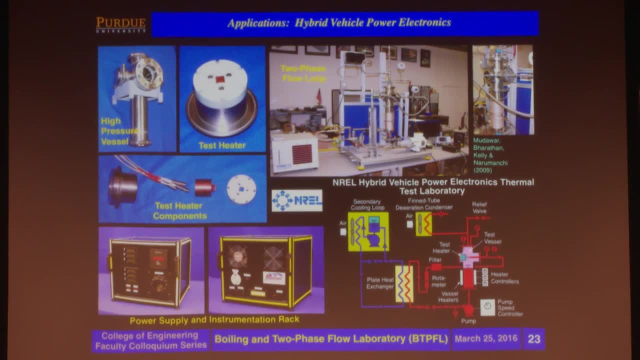 control the temperatures in these applications. And these are the variety of instruments. Actually, they were all built in the research park and they make up the thermal lab right now at NREL. And, by the way, the engineers who built this are all ME students, former ME students. 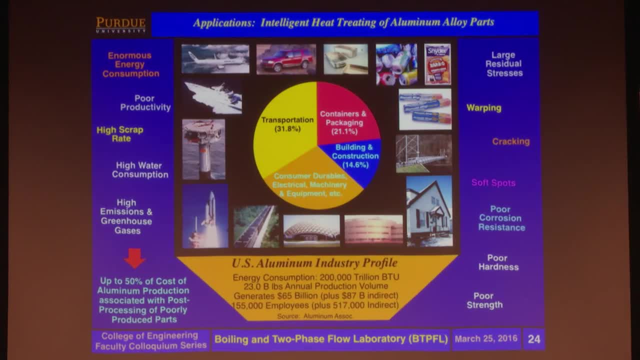 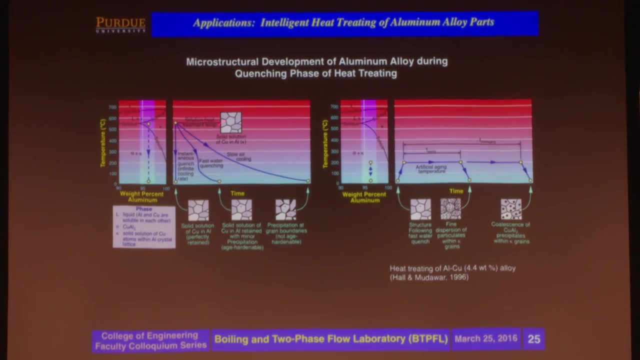 Now, one important application I always like to highlight is materials processing. How boiling is also important in materials processing. I'm using aluminum as an example, but you can apply it for steel, for any other alloy. The idea here is summarized in this plot. 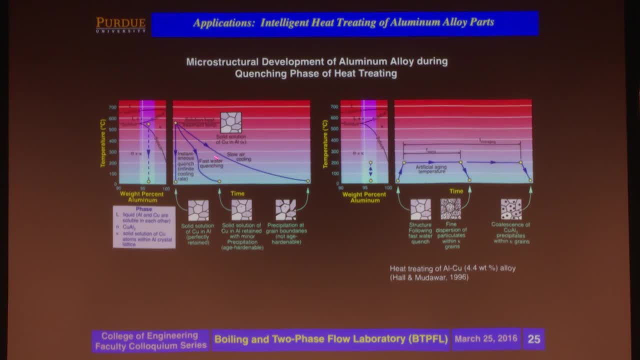 where you take your metal alloy sample, preheat it to a temperature close to the melting point, And then what you want to do is quickly quench it down to room temperature, But ideally freeze the microstructure that you had before so that you can reheat it. 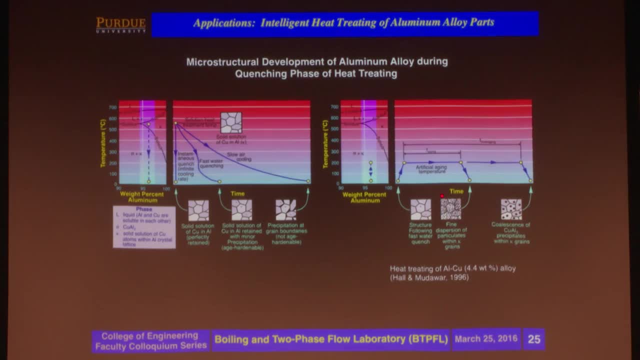 in subsequent process. in order to produce this behavior, You have hardening solutes dispersed evenly throughout the crystals. Now that requires very careful manipulation of the quenching process and the aging process If you don't do the quenching properly. 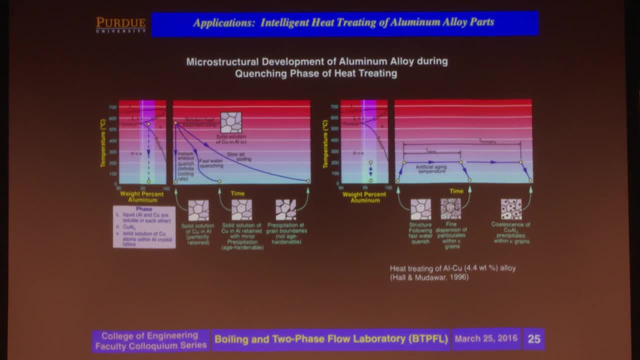 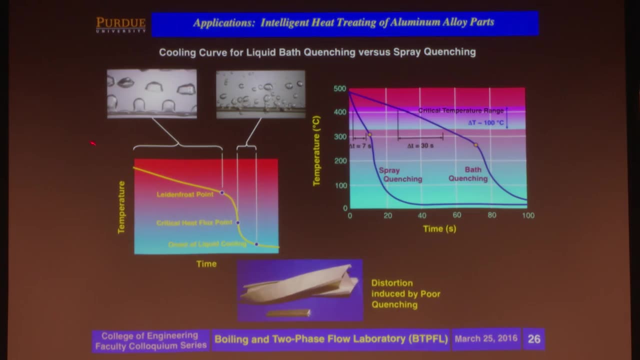 it's going to be a total mess. It's a useless. It's a useless alloy. Now I'm borrowing the same pictures from before to show you how, in what we have here is temperature versus time, what happens as the quench proceeds. 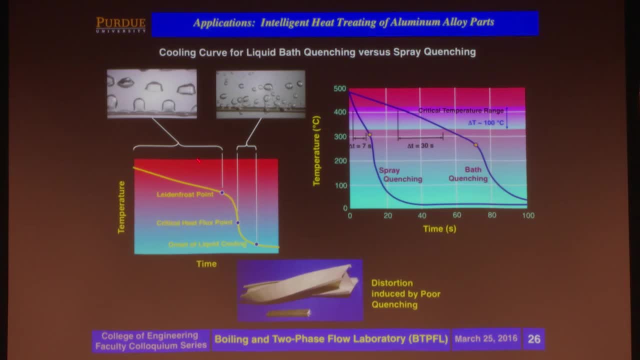 And what happens typically in most operations. I've actually designed a lot of aluminum plants, heat treating plants, And what you see in many cases is how they bring a lot of parts, different shapes and sizes, and throw them in a basket and put them in a bath. 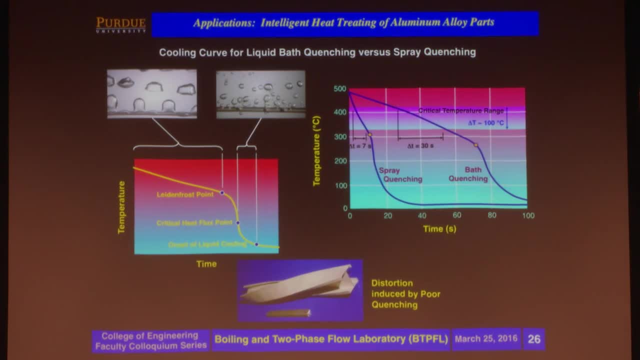 There is absolutely no control over the cooling process. You get distortions cracking And they live with that sometimes, Or they throw away the parts that are deformed more and they keep the good ones, And this is really the type of shape that you get. 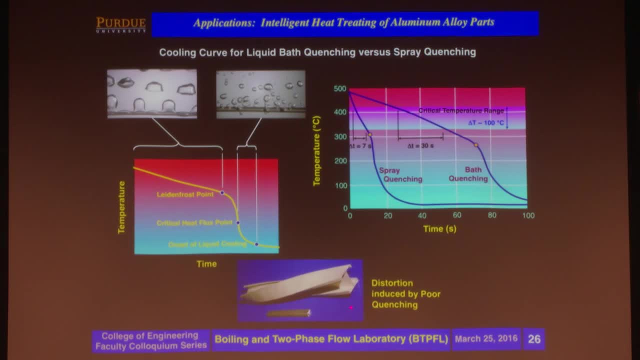 This is about two feet in length And you can see an H shape, completely distorted as a result of poor cooling. So what we're doing is replacing this, what we call bath quenching, with far more effective spray quenching, not only to speed up the quenching process, 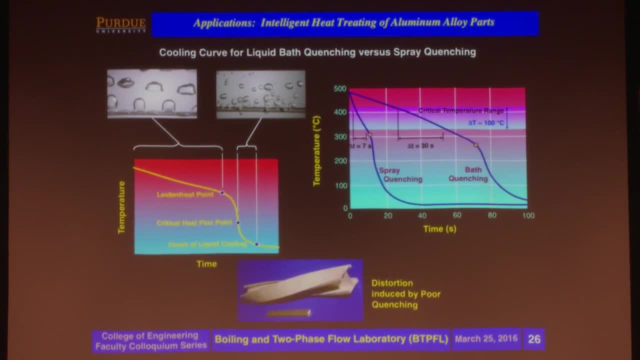 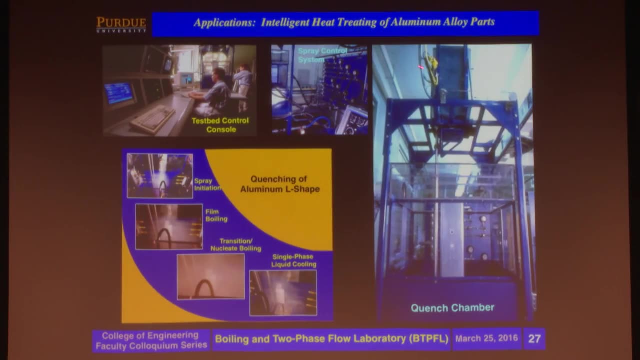 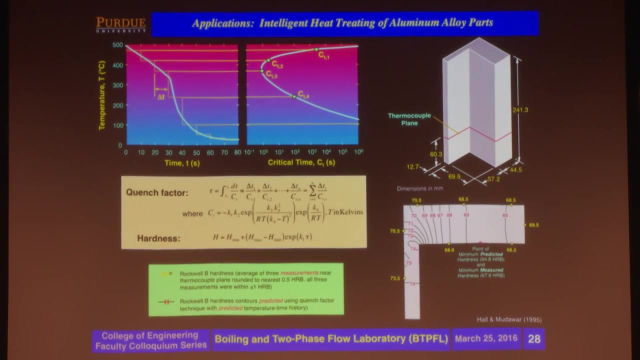 but also to achieve control, as I'm going to show you, And we built a test bed for this purpose, where we have a furnace And we bring the part after being heat treated and quench it within this chamber that you see right here. 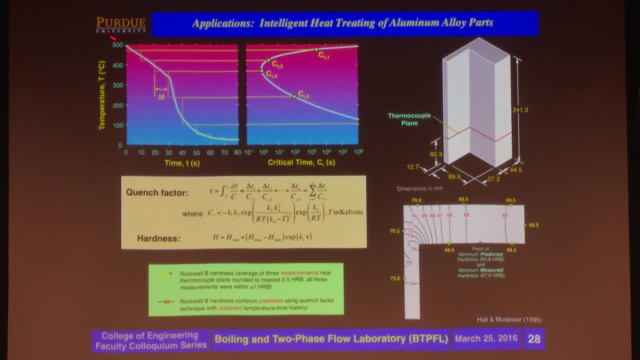 And what we were able to do is combine our understanding of the quenching process with metallurgical transformation theory in order to optimize the impact of the quench on the material properties, namely hardness and strength of the part. So, by this optimization process and changing spray boundary, 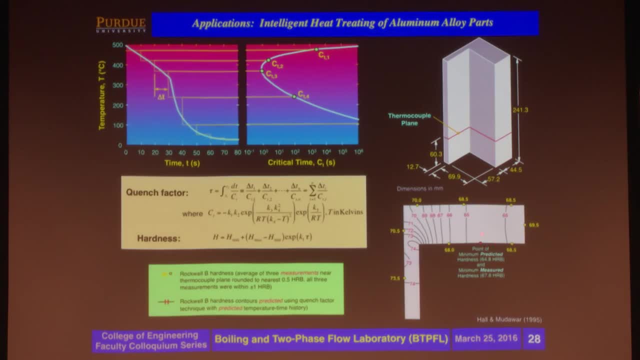 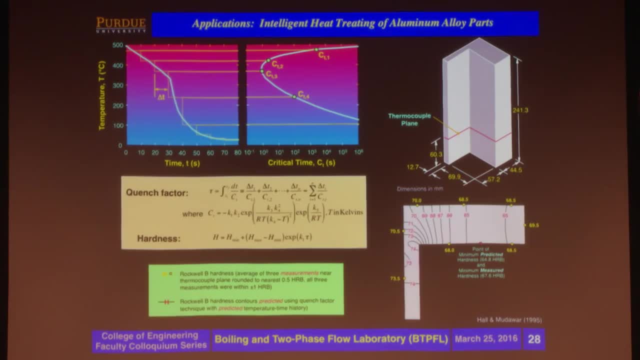 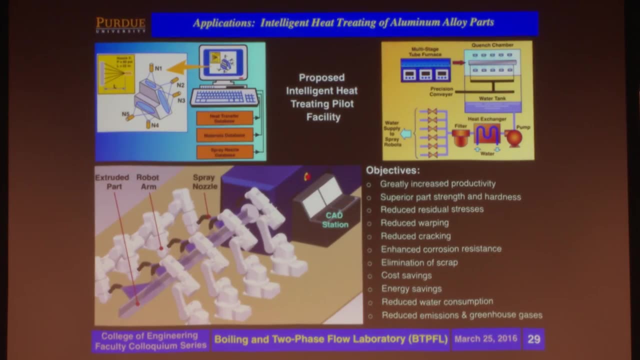 You don't have to run experiments by trial in order to achieve this result. Ideally- and that's something I've been trying to promote and I'm talking to different people to do- it is to do all of this robotically, by having robots lined up to quench the part. 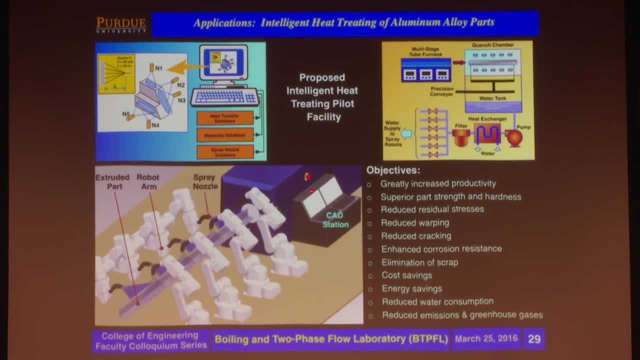 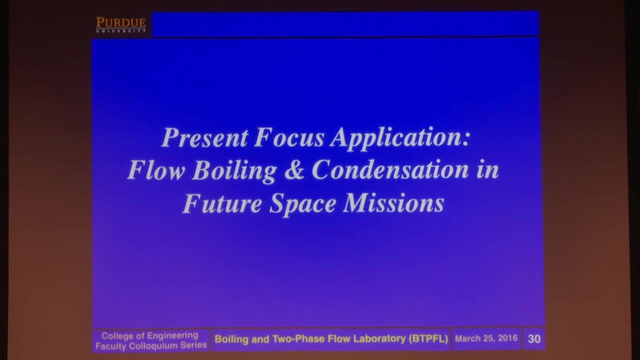 from all directions, based on predictions from a CAD system. Now, another area I want to talk about, which is really the primary focus for us at the present time, is flow boiling and condensation for future space missions. This is a NASA-funded effort. 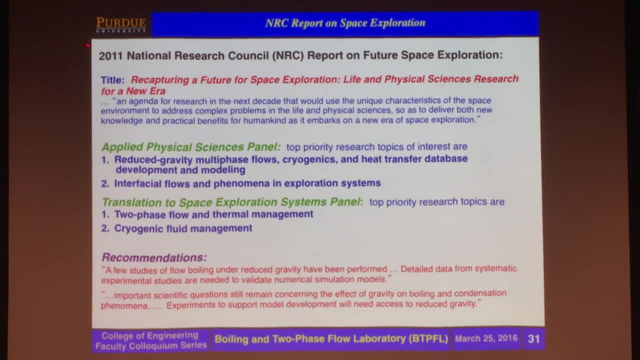 And I just want to mention that in 2011,, a report came out from the National Research Council on Future Space Exploration and presented to the Congress and with recommendation from a combination of national academies, science, engineering, et cetera- regarding space exploration. 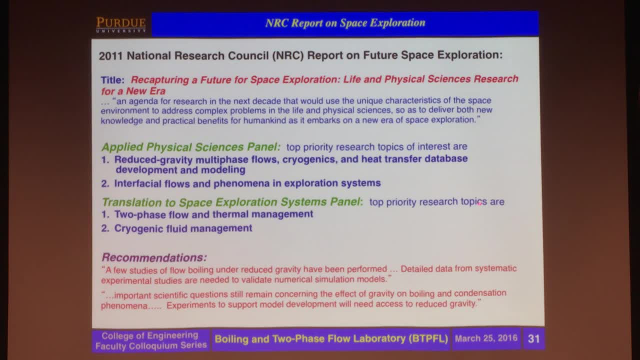 What fields of knowledge are needed to achieve the goals NASA has set forth? And when you look through the report, it's a very thick report. But section after section, you see a repeated mention of phase change as a primary area of research. Why? 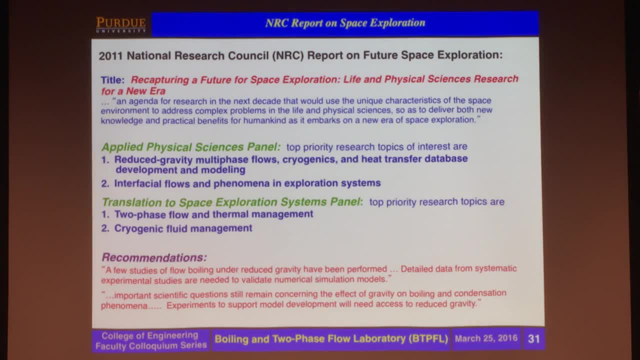 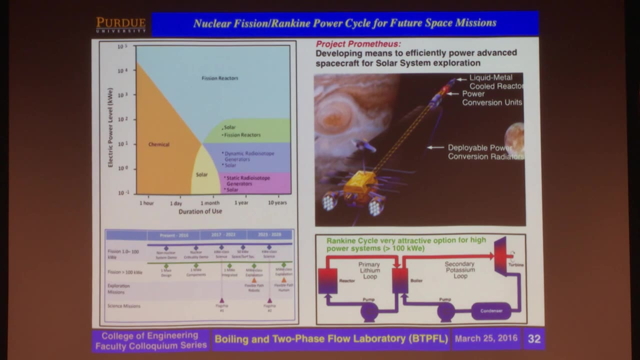 Because with phase change, you get better heat transfer. With better heat transfer, you have smaller area devices, more compact, lightweight, which is ideal for space applications. And here are some examples where phase change becomes really important: High-power space mission, long-duration space missions. 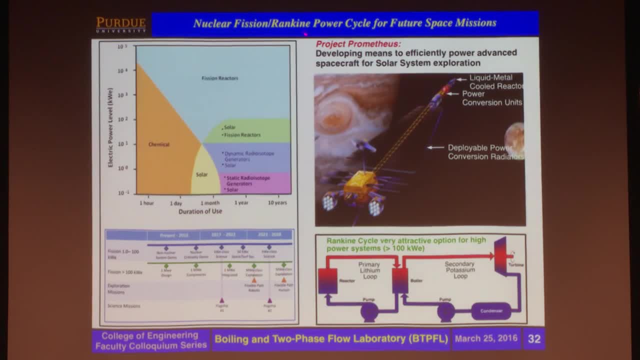 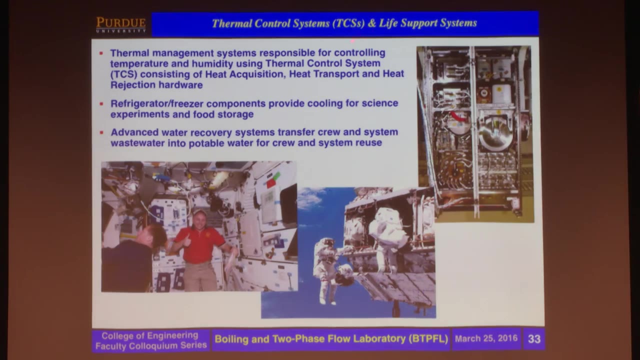 will require fission reactors. Recently, Project Prometheus talked about using also a reactor with liquid metal boiling and condensation. A more immediate application is Thermal Control Systems, TCS, And we are really heavily involved in this. This is what is required to control temperature and humidity. 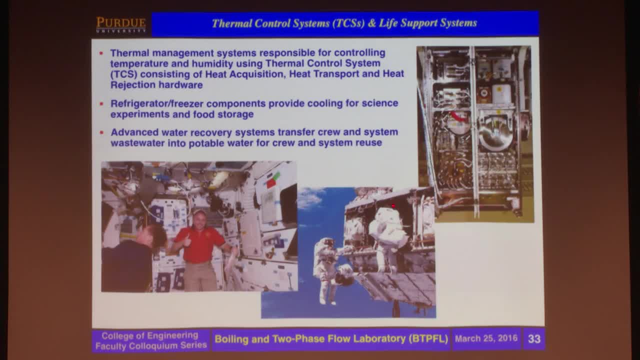 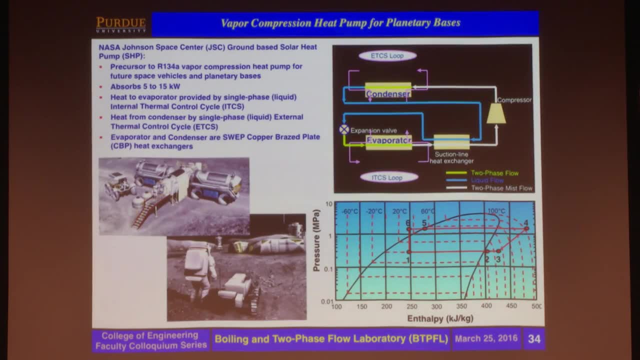 on board the space vehicle for the comfort of both electronics and crew Very, very important. Another area is vapor compression heat pump for planetary bases. This year There was an announcement from the government that NASA should refocus on planetary habitat And temperature control is achieved. 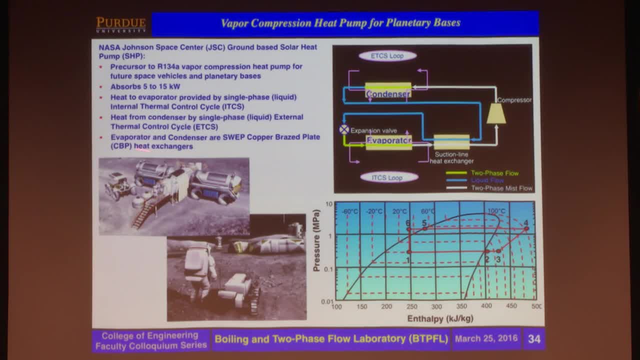 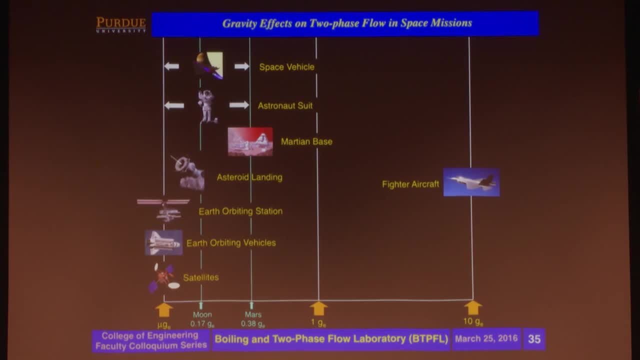 at the level of about 40 kilowatts now with Martian habitat, with systems like ones you see right here. So in our research we looked at the various applications And we found that you're not just focusing on microgravity. We obviously know a lot about the one. 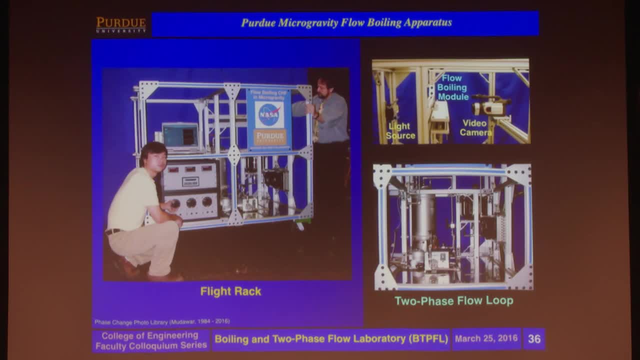 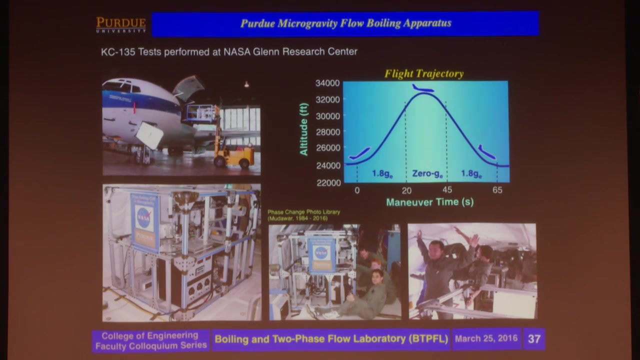 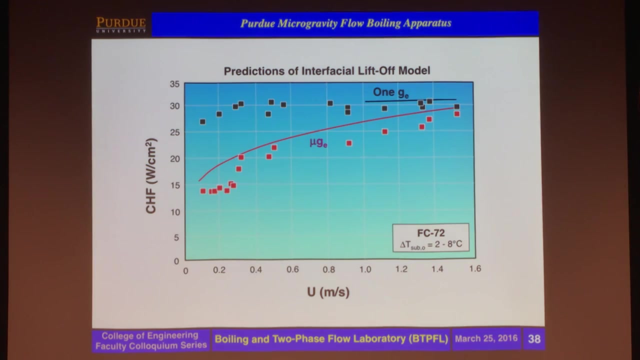 So around 2004, we did our first study related to microgravity phase change. We built a flight rig for flow boiling in microgravity. This was flown on a couple of occasions using KC-135 aircraft and NASA Glenn And it produced- this is a plot NASA uses quite a bit. 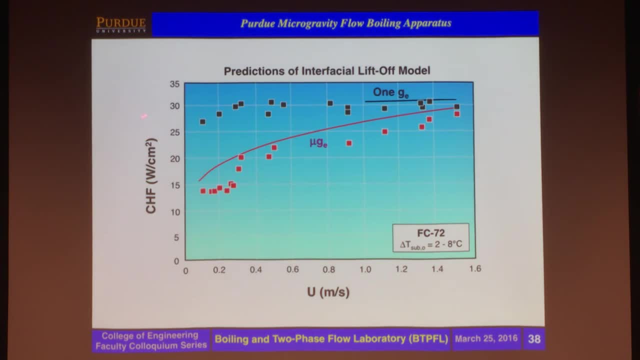 from our data. It produced this plot of critical heat flux as a function of fluid velocity And showed how at very low velocities you've got to be really careful about the effect of reduced gravity- And you can see that in microgravity- on critical heat. 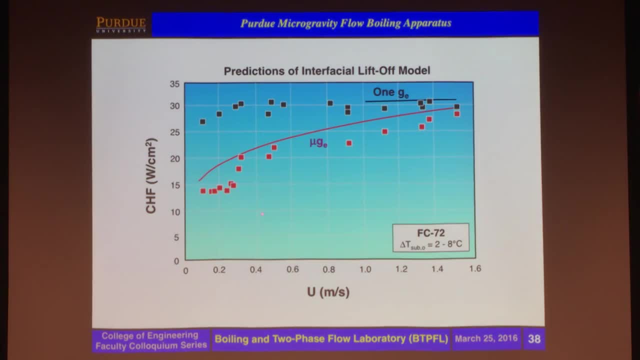 flux, you really compromise cooling tremendously compared to 1 G. However, it also shows that at certain velocities the inertia can completely overcome the down effects of microgravity, And this is very important because it tells you you would rather operate at this condition, right here. 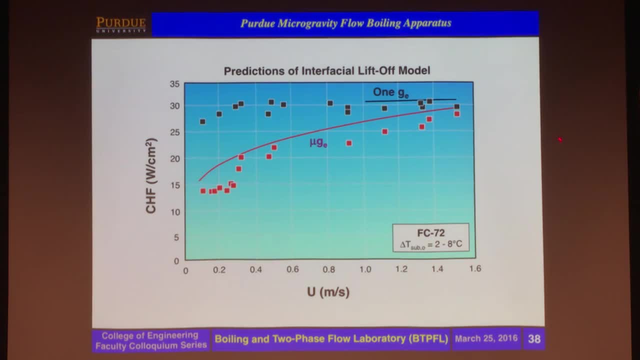 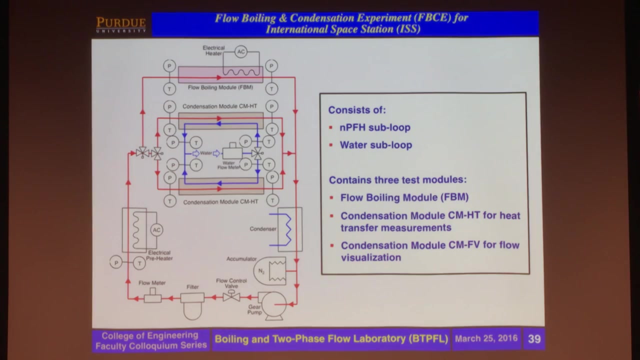 You don't have to operate at much higher velocities because you're losing energy- OK power dissipation- here in the pump. So this conversion value is extremely important. And nowadays, since 2012,, we received a contract to develop the flow boiling and condensation experiment. 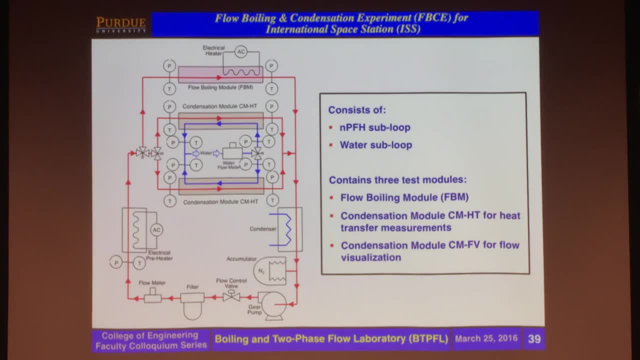 FBCE for the International Space Station. Two months ago, this was announced to be a very high priority project for NASA now And we have literally over 50 scientists and engineers from NASA Glenn supporting this project. So it's growing and it keeps growing. 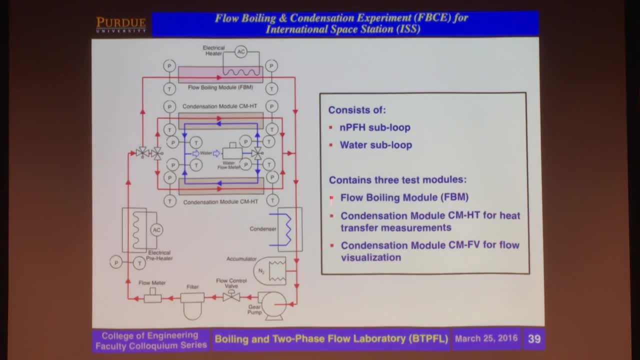 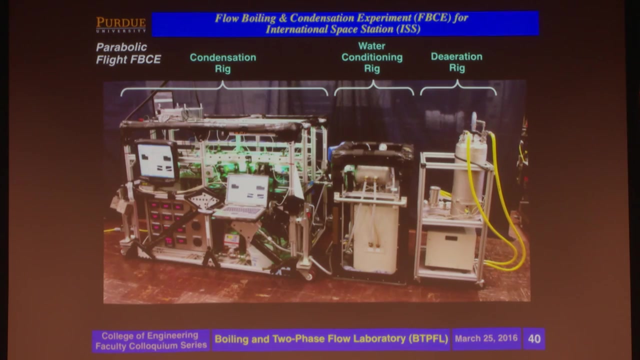 And the idea behind it is to develop a very complicated flow loop loaded with instrumentation and high-speed video to investigate both flow boiling and condensation using three test modules that you see right here, And we quickly developed a test rig- flight test rig for condensation, because we had not done any work in this. 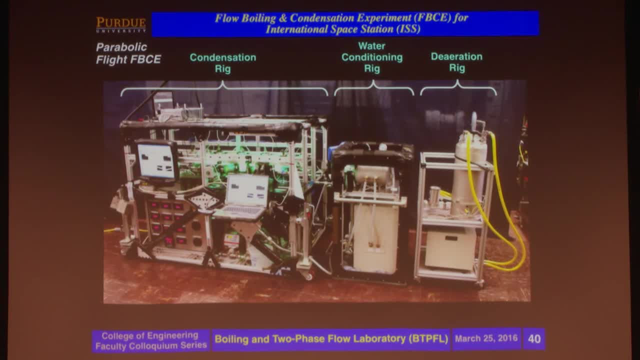 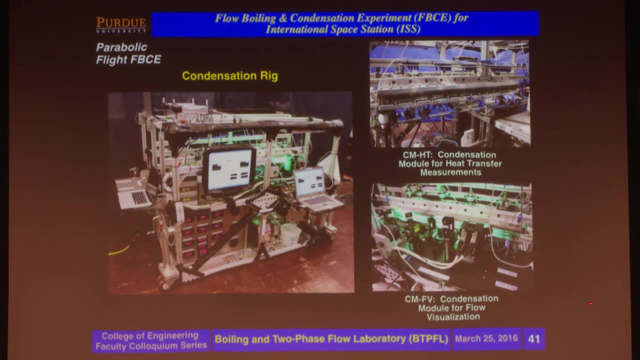 And nobody has done this type of work before. And this test rig- we built it here at Purdue- has two flow channels. As you see, it's loaded with instrumentation, pressure, temperature, high-speed cameras everywhere, And it requires six operators dealing with various aspects. 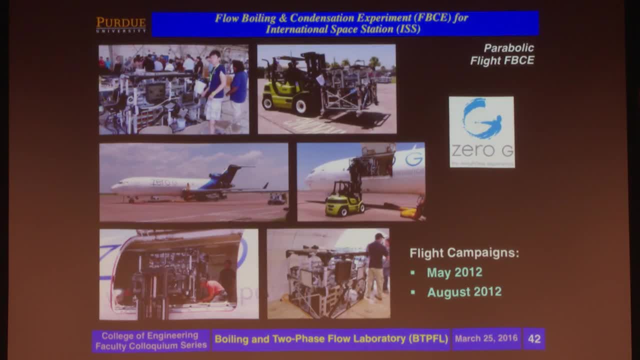 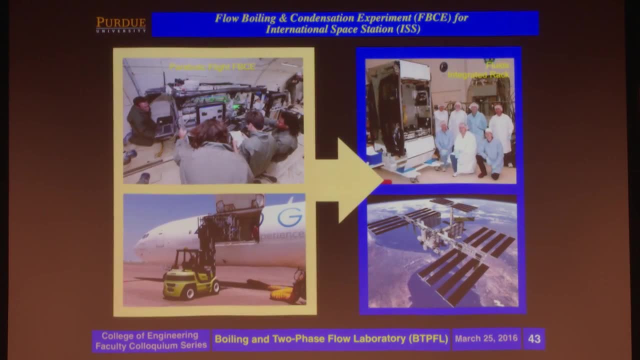 of the experiment And we flew that on a couple of occasions using zero-gravity air and zero-gravity aircraft. We had several students actually participate in this effort, And where we're at right now is really shifting attention to the integration into what's called the fluid integrated rack. 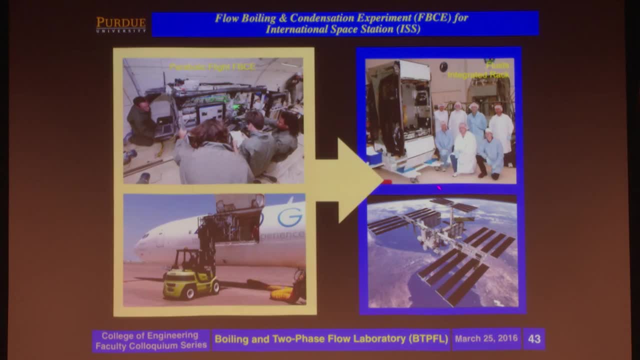 This is a replica of the system available on the ISS. This is the largest setup available to run fluid experiments And we're trying to package all our hardware in an area in a space about one meter by one meter, but maybe about less than one meter depth. 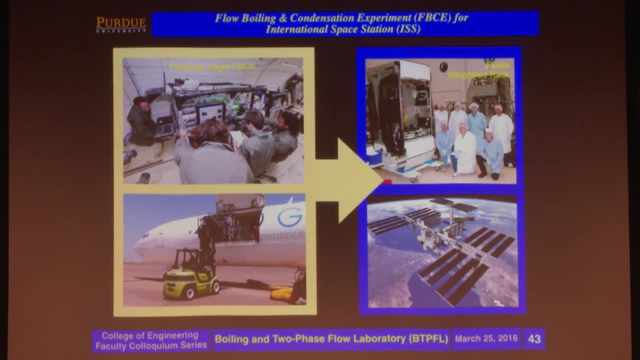 Okay, all this instrumentation has to be converged, So we're due to transport the hardware for this application in two SpaceX flights, hopefully Tentatively. this is what's scheduled right now, because there's a lot of hardware involved over the next few years. 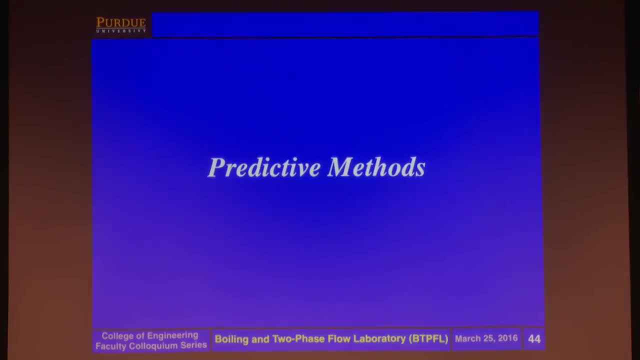 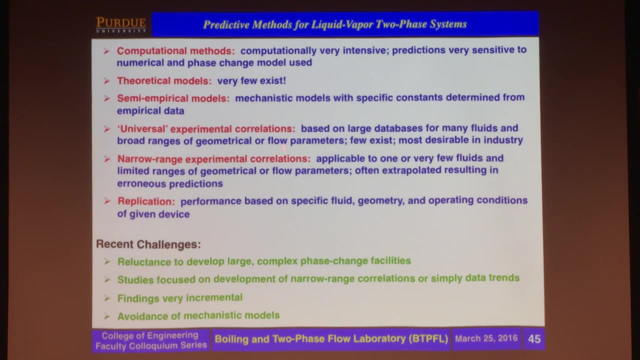 Now I want to shift the attention to talk about predictive methods. talk about the theory a little bit. This is probably a very important chart in the sense that it summarizes what people have done over the years in regards to predictive methods in boiling and two-phase flow. 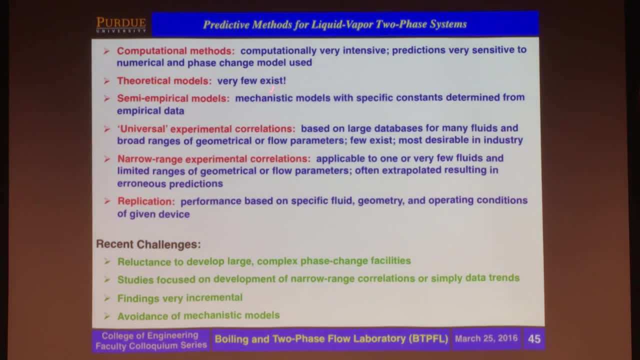 Now, ideally, you want to have convenient computational tools to do that, but you find that these are not very effective at the present. Depending on the tool that you use, you get different results. You get different results all the time. But it's very important because that's going to be the next step in a lot. 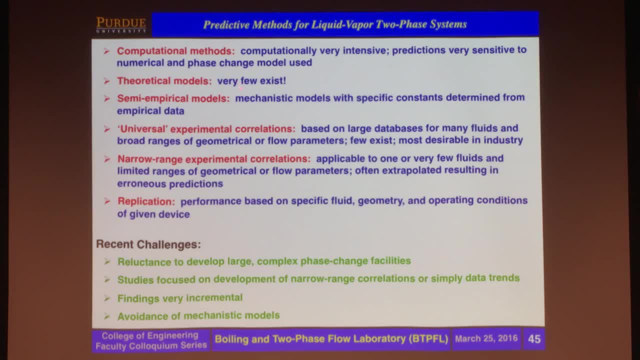 of the predictive approaches that we're going to use: Theoretical models: very few of those exist in the two-phase literature. Next, semi-empirical models, meaning models based on theory, on mechanism, but they lack closure. and that's where you fit the model. 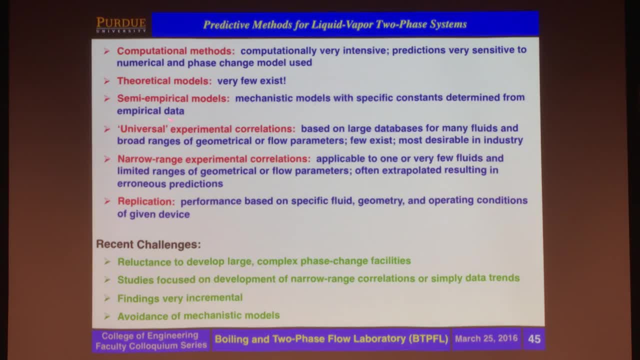 with empirical constants. The next step is universal correlations. These are correlations that are developed based on enormous databases for many fluids, many geometrical parameters, many operating conditions to give confidence in the predictions. Then you have narrow-range experimental correlations. This is where, if you look at the two-phase literature, you find a vast 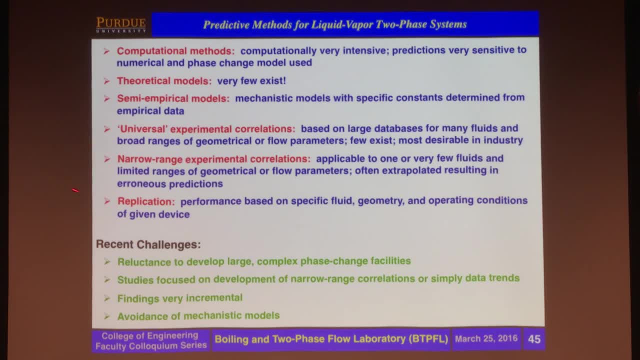 majority of literature focus on this approach right here. And this is very dangerous because what you're doing is obtaining 10 data points for one fluid and one geometry and saying I've got a correlation to predict the flow And I'm going to show you why this is very dangerous in a minute. 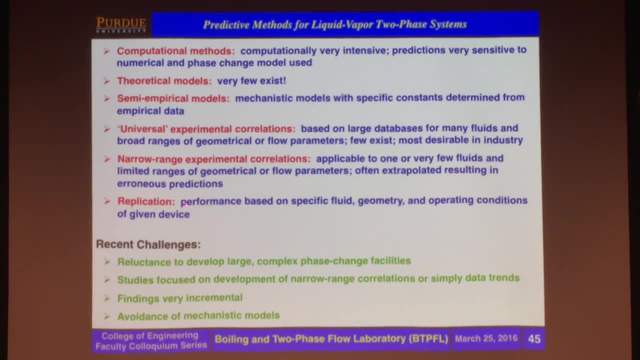 And then replication is used by some companies, just by testing a particular device at a particular condition. If it works, it works, We're happy with it. Now our approach is to use those fluids, The first four, we have been using those three and now we're just beginning. 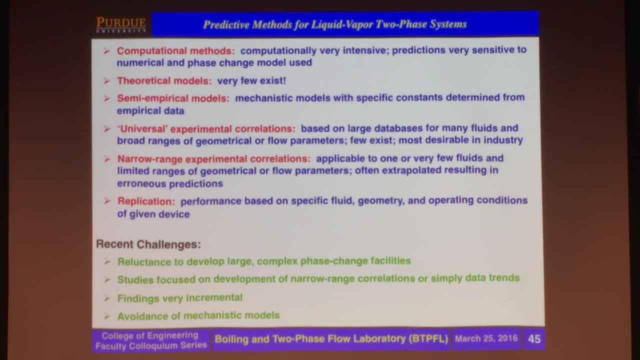 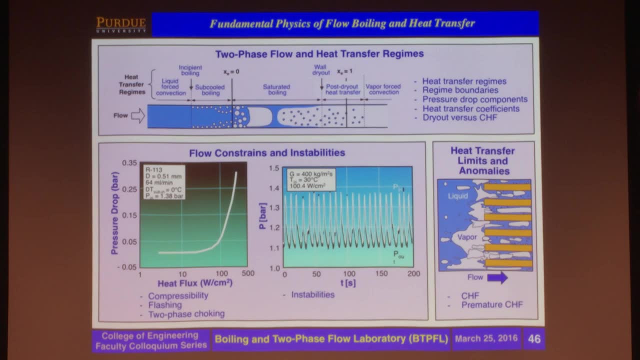 to converge on computational methods. Now, just to show you why it's very complicated to model two-phase flow accurately, I picked the simplest geometry by far in two-phase flow, which is flow boiling in a tube, circular tube. Now to be able to predict heat transfer behavior in a situation like this: 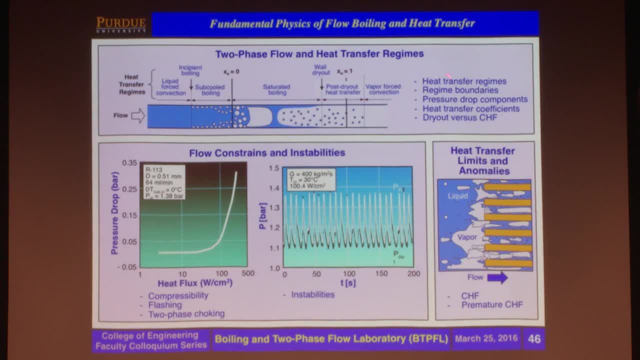 you have to know many different things: Heat transfer regimes, regime boundaries, pressure drop components, heat transfer coefficients, the limits of dry out, for example. Also, you have to appreciate the flow constraints. For example, you can have a lot of compressibility. 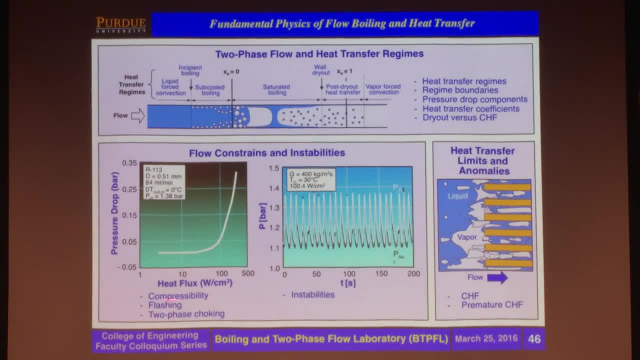 You can have a lot of flashing due to latent heat effects. You can have two-phase choking. You also have a lot of potential instabilities taking place in two-phase systems, so you have to be mindful about those And ultimately you may hit critical heat flux and reach burnout before you know it. 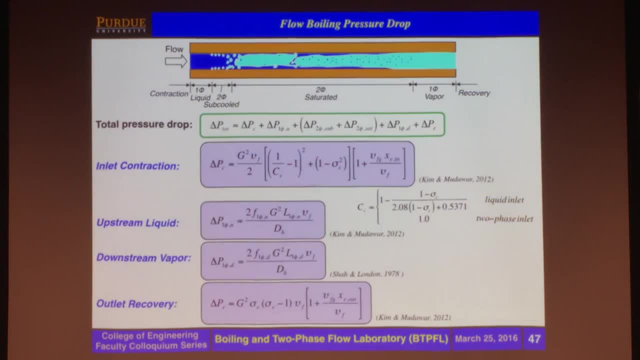 So you have to really be concerned about all these aspects simultaneously, which is why, to do a good job with those predictions, you break it down very, very carefully and make sure that every component is handled properly, And these are some examples of those. 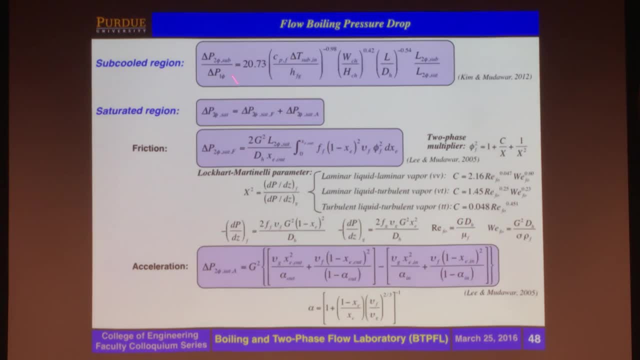 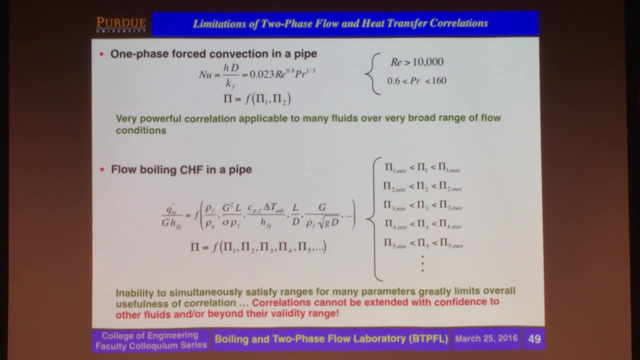 The most critical components are the ones where there is both vapor and liquid. obviously- And this is also important because it explains why it's really vital to have what I call universal correlations- If you compare, for one-phase flow, a very simple correlation for heat transfer coefficient: 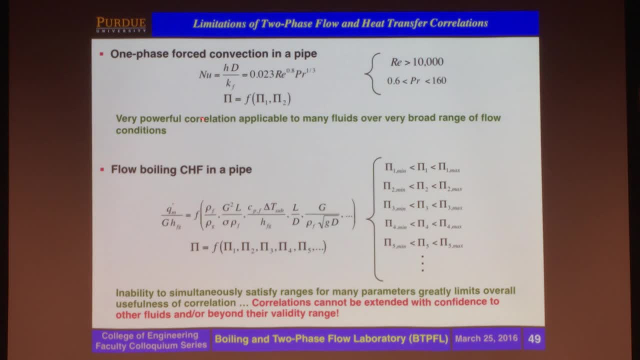 as a function of Reynolds and Prandtl number, you find that you have three dimensionless parameters, two independent parameters with fairly broad ranges of for both. This is a very powerful correlation and very easy to use. If you look at the counterpart, for example, flow boiling- critical heat flux in a pipe- 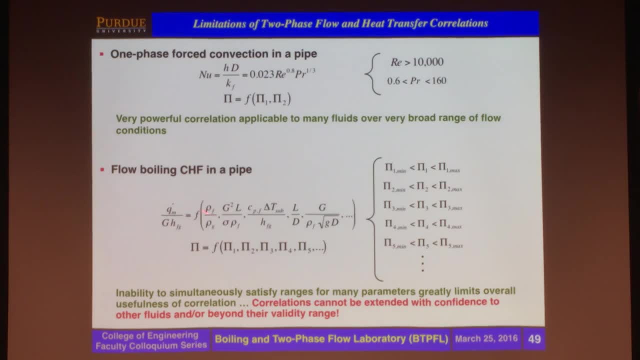 you find that you have a dimensionless group that may be a function of as many as nine or ten dimensionless groups, And each one of those is confined within limitations imposed by the experiments. And because these experiments are very expensive, it means those are all narrow ranges. 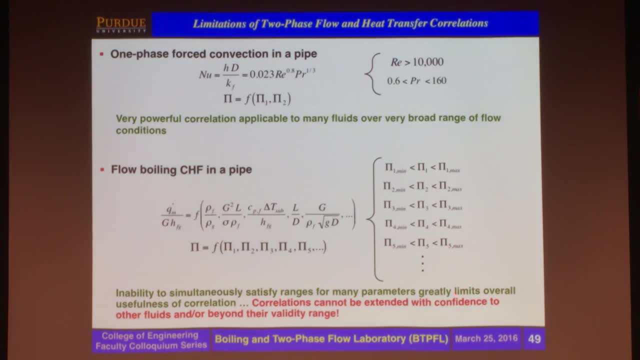 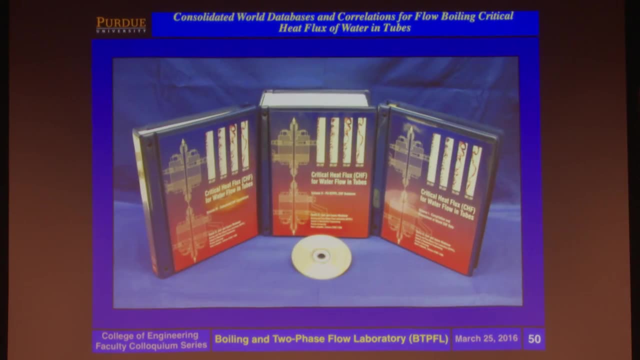 So it's very, very difficult to achieve universal correlations. You have to be very patient and work very hard to get that kind of formulation Now. we knew that for a long time and we tried to go in that direction. So back- that was in 1999, we were able to consolidate the water databases. 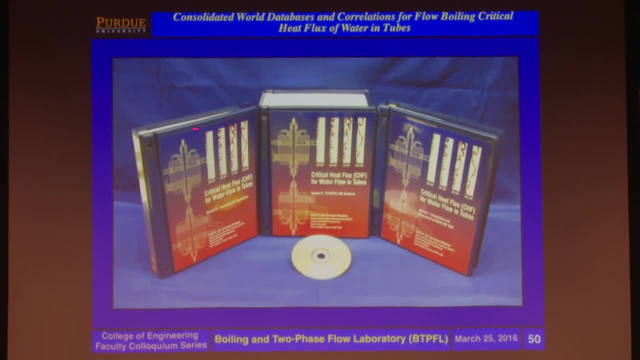 This is for nuclear reactors. We went back and obtained literally every data point you can find anywhere And it took us about five years of search with the library help to put it together and develop universal correlations. but they were still for water alone And then we started doing it for mini and micro channels. 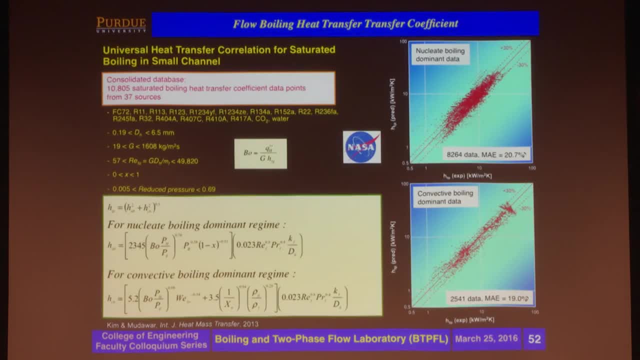 because that's a technology that is very important nowadays, And in the last three years we developed a series of studies of truly universal heat transfer correlations for small channels, for heat transfer coefficients for pressure drops, for condensation, for adiabatic flow and for dry out. 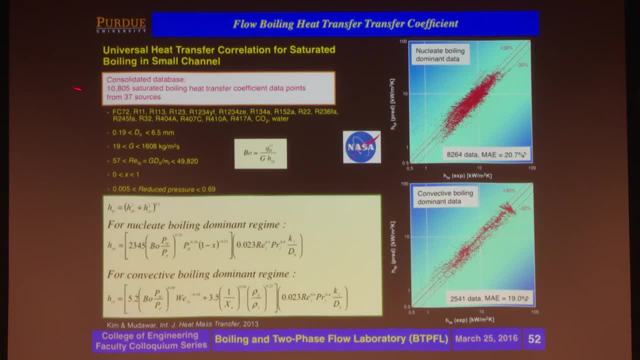 And you could see how we did that. It's large databases obtained for all the possible fluid. we found in the literature broad ranges of operating diameters and pressures up to close to the critical, And people have started using those correlations And they're extremely accurate because of the universal appeal. 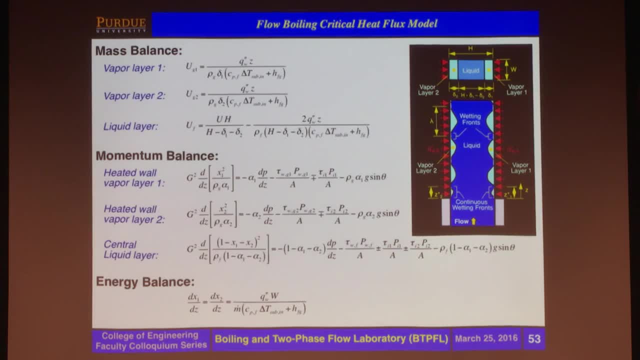 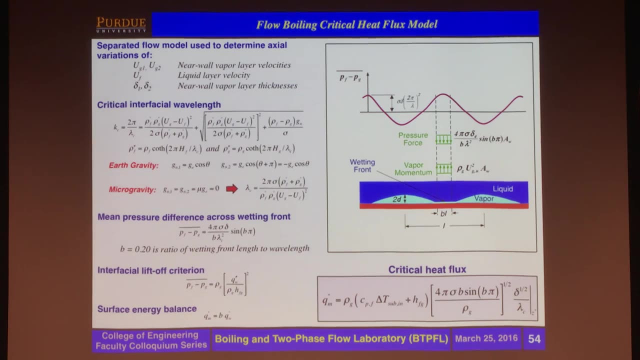 We also have been doing a lot of theoretical modeling in the form of proper use of conservation laws for two-phase flow, such as here, flow boiling. critical heat flux- theoretical model for critical heat flux, which, as I said, is the most critical point for boiling. 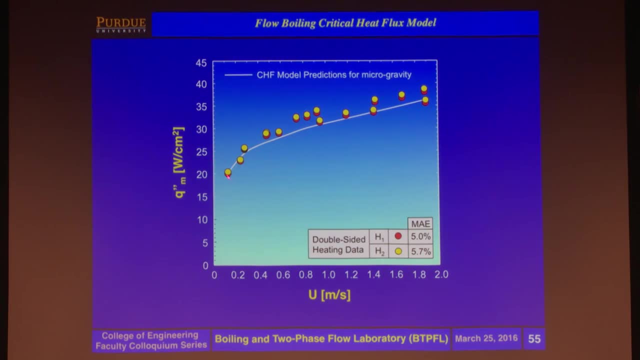 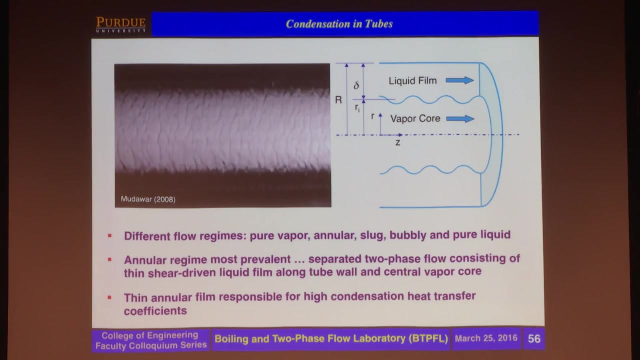 And we are able finally to come out with very accurate predictions for, particularly for microgravity, because we're very interested in this for the application of future space flights. Now, another application is condensation, which is flip side of boiling. Here, what you're doing is rejecting the heat. 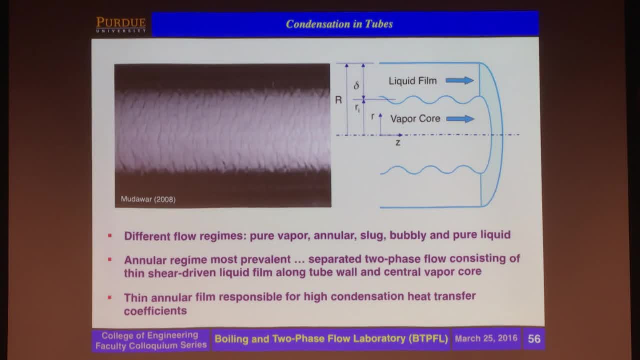 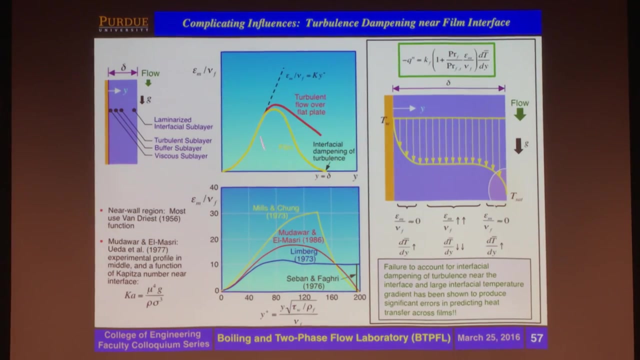 by condensing the vapor back to liquid. The liquid flows on the inside of a tube along the wall surrounding a vapor core, But the flow, even though it's separated, is very complicated. One of the complications is what happens at the interface. 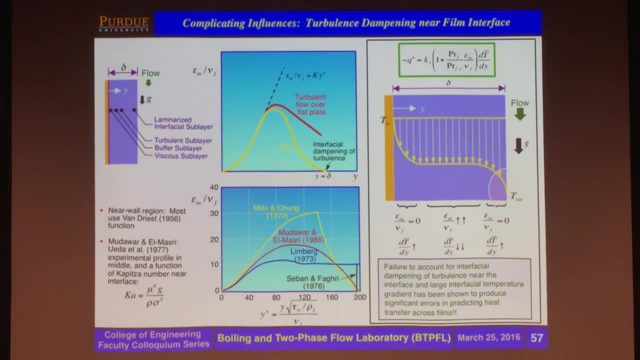 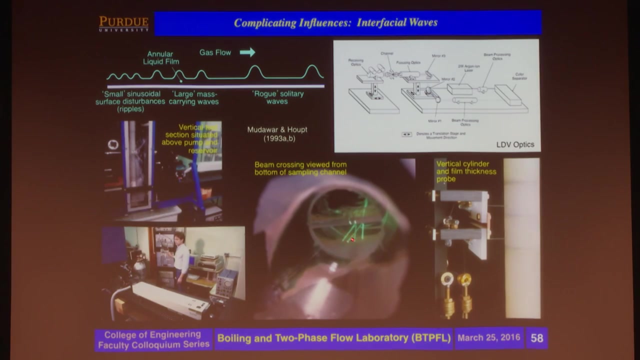 We found that there is significant dampening of turbulence taking place at the interface because of surface tension, which is something you don't encounter in other types of flows. So we had to model this effect very carefully. We also did LDV measurements of flow and turbulence. 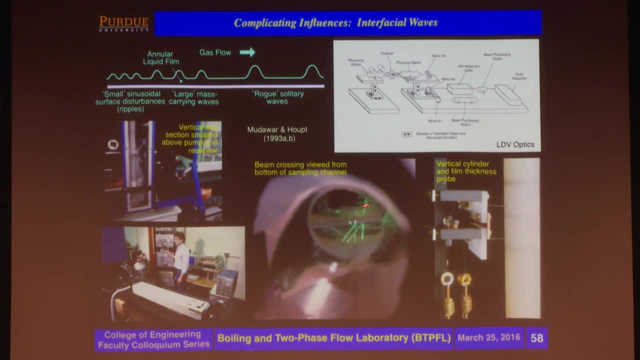 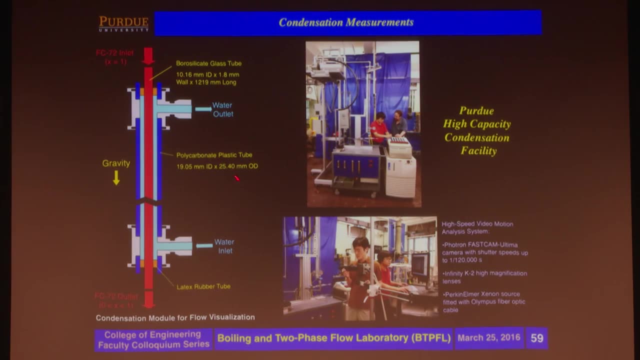 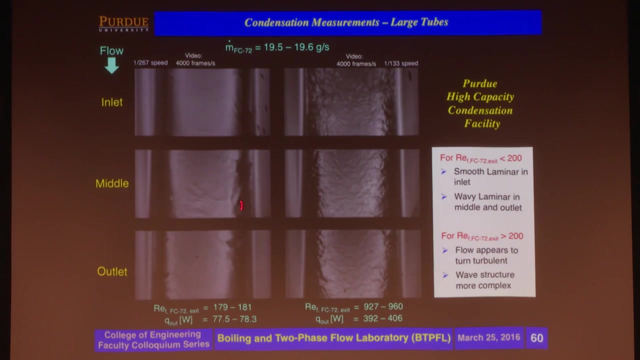 within a liquid film. We did that extensively. Then we built several facilities related to condensation at different orientations relative to gravity, And the goal was to try to identify the flow mechanisms, particularly the waveness that takes place along the interface, which you see here changing drastically. 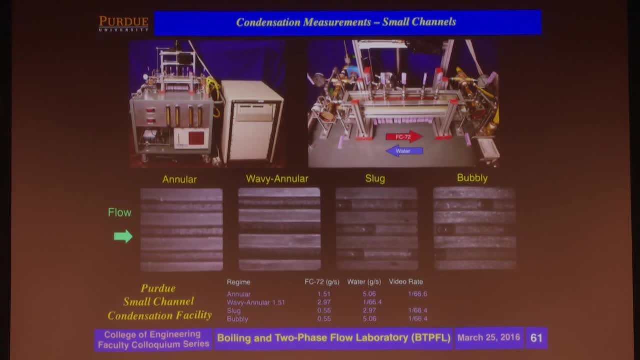 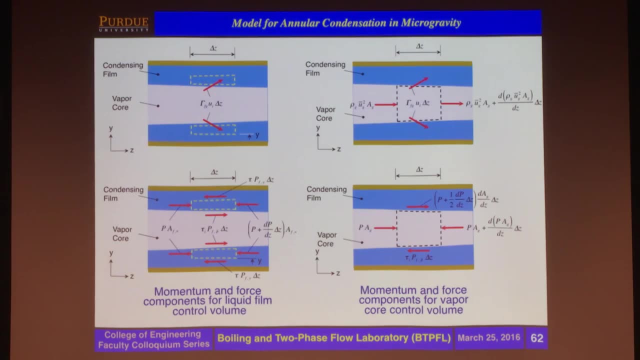 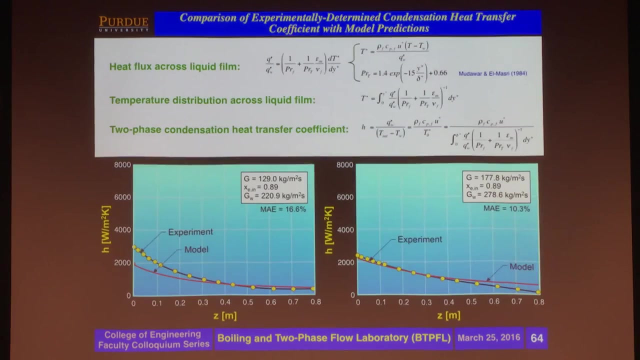 at low Reynolds numbers versus high Reynolds numbers. We did the same for many channels and micro channels, And also we developed control volume models for condensation, which combines with the added diffusivity profile I just mentioned. We are finally able to make good predictions. 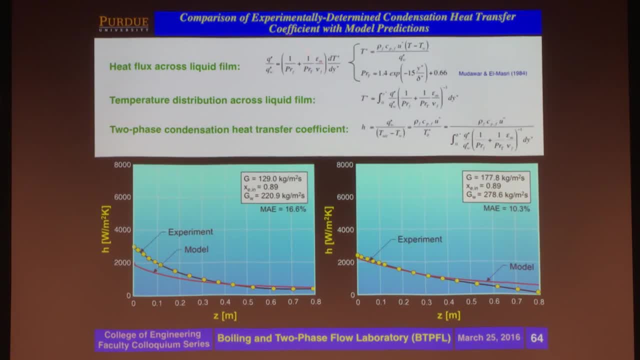 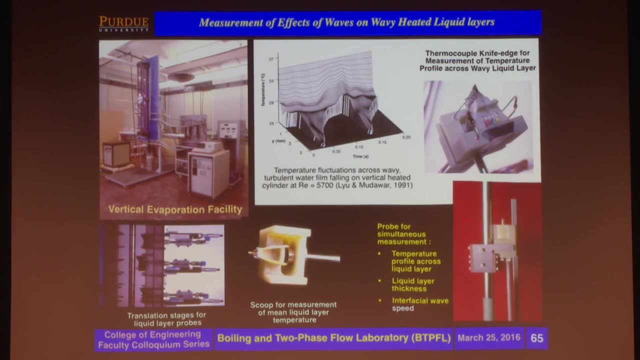 for condensation in microgravity. So NASA is actually using those right now for space applications. Now we also did the same thing for falling films involving evaporation of liquid films, With specialized probes that are capable to simultaneously measure film thickness, velocity of the waves. 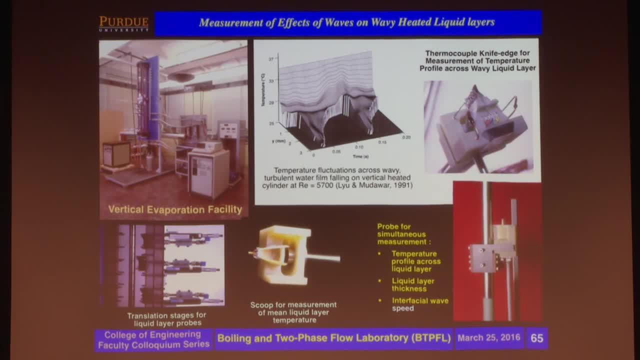 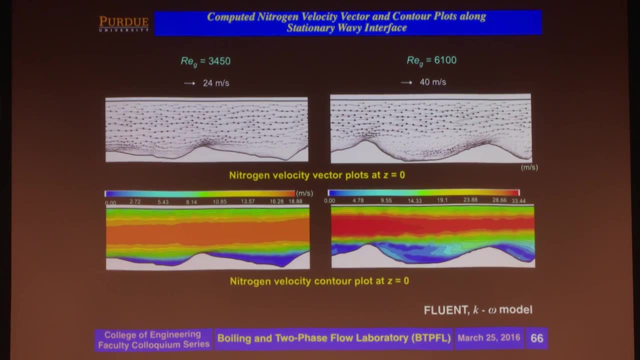 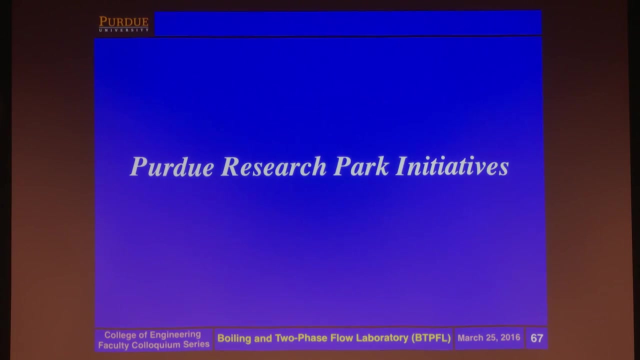 and temperature profile within a liquid film. all at the same time, And also very recently, we started looking at what happens around wavy interfaces of liquid films, which is what's shown right here, And so looking also at research park activities. 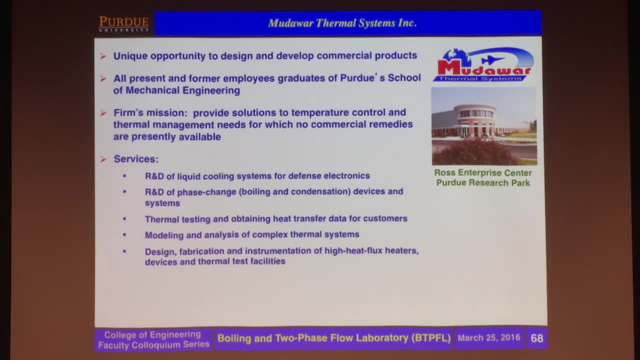 I was mentioned earlier. I wanted to mention this for you: What it is to start a company at the research park. to me, it was very important because it's a unique opportunity to develop design products, actual products, something we cannot do at the university. 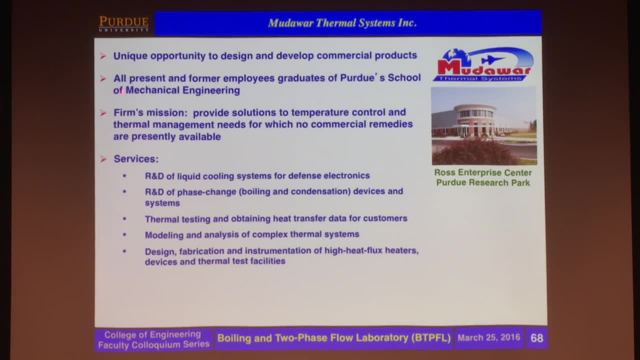 And, as I said earlier, all the present and former employees are Purdue grads. because you need the ME, particularly Purdue ME students, because you need that kind of expertise And the mission statement is to provide solutions to temperature control and thermal management needs for which no commercial remedies are presently available. 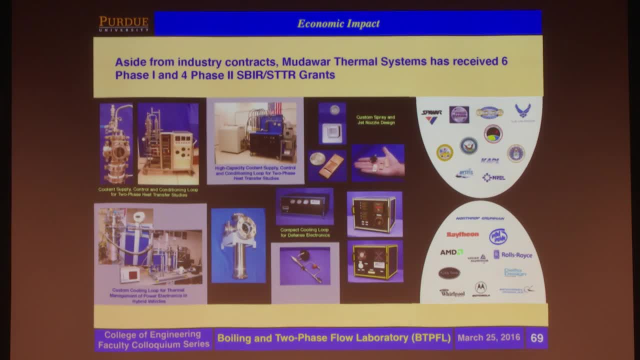 in a nutshell, And we have received over the years, aside from many industry contracts, six phase one and four phase two SBIR projects. I don't know if you know about phase one versus phase three. Phase one is like they give you up to 100,. 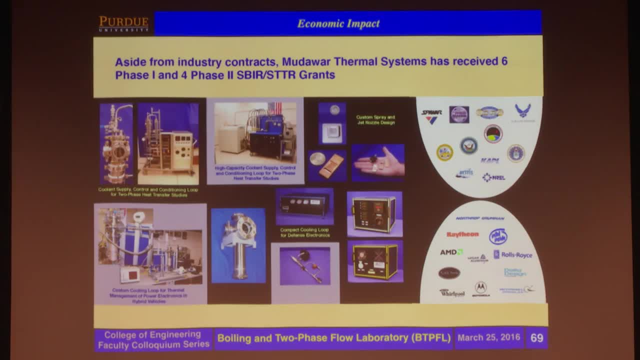 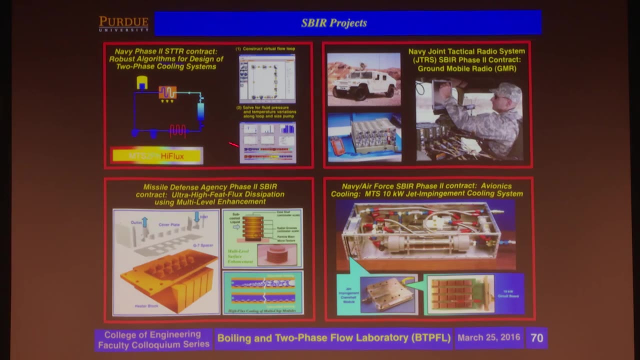 $150,000 to get started Phase two. they give you a million dollars to go beyond and do the verification And you can see here the variety of products produced and testing capabilities. And these are some examples of the different projects: CAD-based predictive tools for two-phase systems. 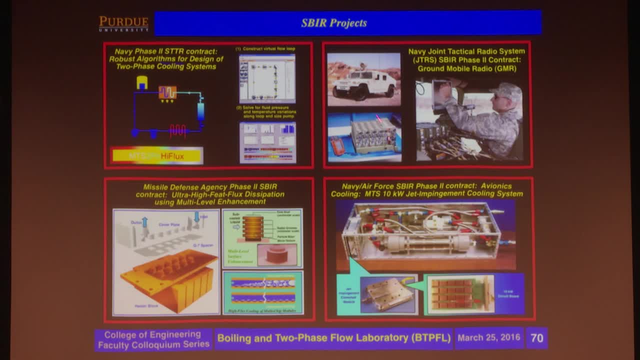 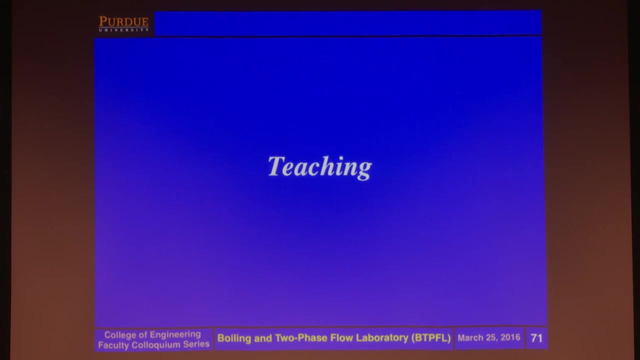 ground mobile radio thermal management, boosting the capability for that, avionics and ultra-high heat flux devices for extreme heat dissipation. Now I'm almost done, by the way, Teaching. you know I have just a few concluding slides here. 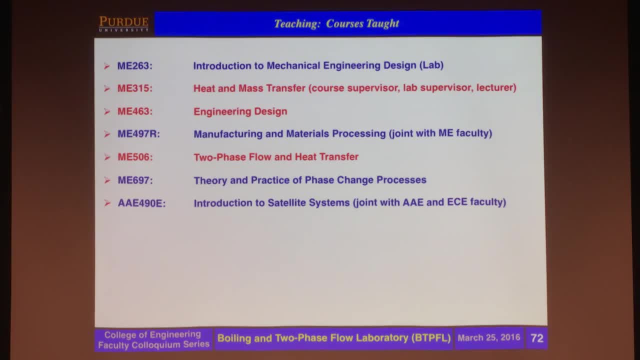 Over the years, I taught these courses that you see here, And the ones that are marked in red are the ones that I spent a lot of time on and a lot of energy over the years: Heat and mass transfer, the undergraduate: 315,. 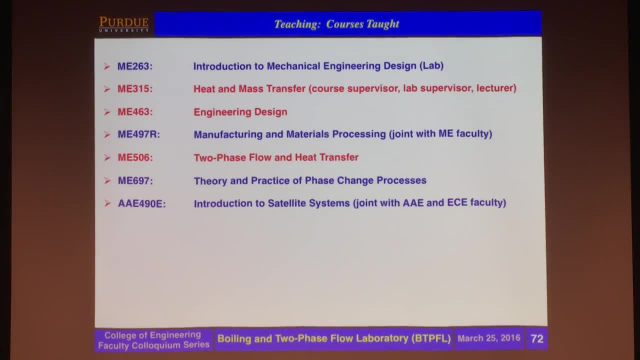 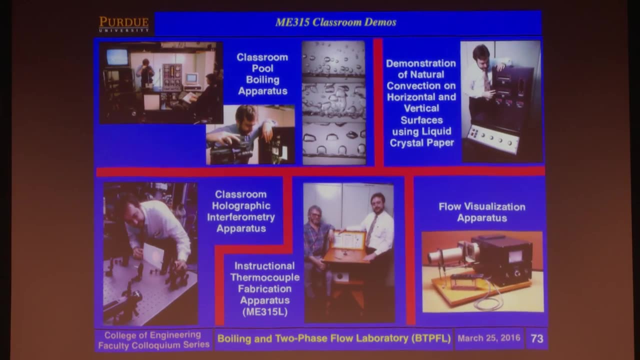 senior design and my two-phase course, graduate course. Now, one of the things I always like to do is introduce lab experiments, introduce the lab to the classroom by running experiments in the classroom, particularly in this room, by the way, for my ME506.. 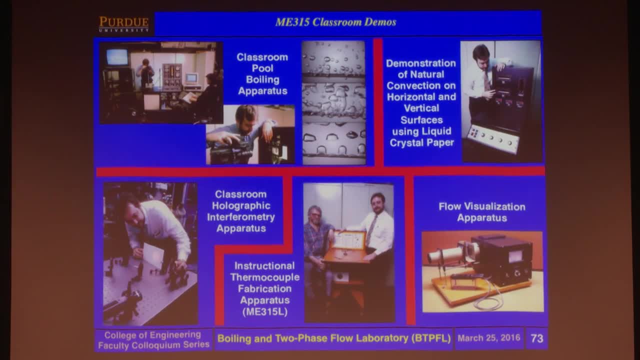 I find it to be extremely useful, particularly for complicated phenomena where you can't just sketch it out, Where you can't just sketch it on a piece of paper. you have to run the experiment live, And it's been very rewarding to do so. 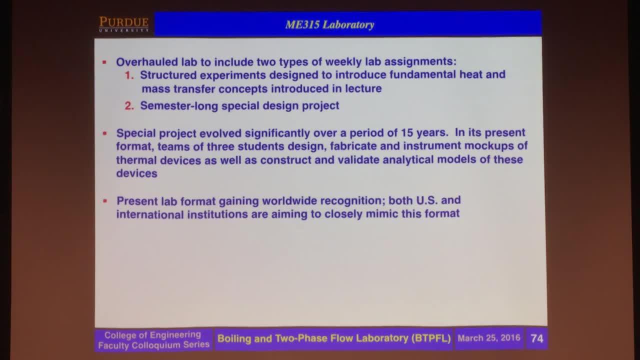 If you look at our ME315 lab, we overhauled the lab so that now what we have is two different components. One of them is structured experiments to help the students appreciate fundamentals, and also a design project where they build a device, instrument, it, model it. 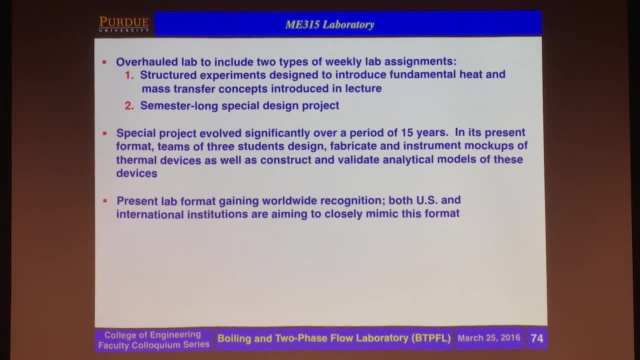 and show the performance and then compare it to predictions. And I should mention, by the way, that this format is very popular worldwide. We're constantly asked by other universities from the US and overseas how to duplicate this format Now. fortunately, we have a huge investment in it. 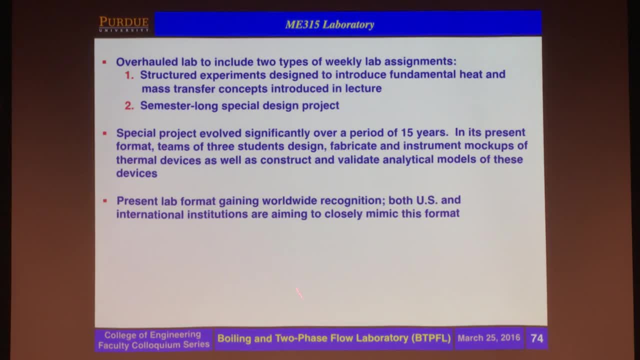 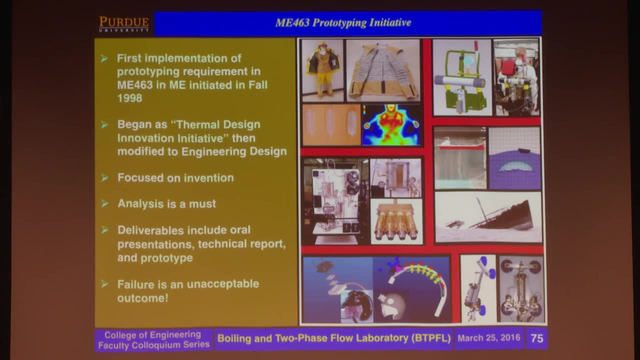 particularly in the form of a lot of TAs manning the effort, but we are very proud of this particular effort. Senior design. I've been involved in every stage of this course, starting with the mid-'80s where it was the worst course on Earth. 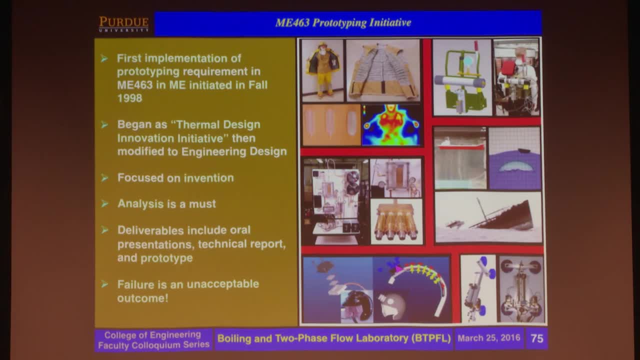 It was an utterly useless course. It's like homework assignments. We call them senior design, literally. So it changed over the years. In the late-'90s I decided to turn it into a prototyping course And I called it the Thermal Design Innovation Initiative. 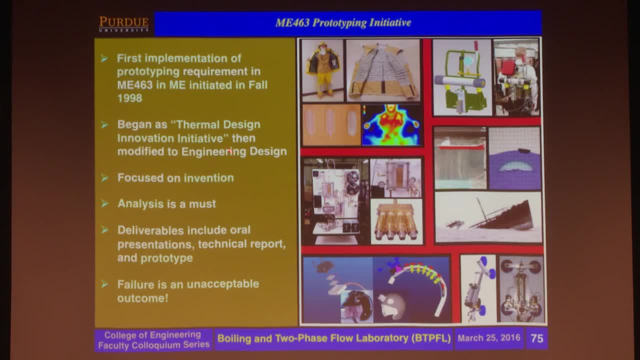 because I was demanding particularly thermal projects for that purpose. The focus was on invention. The students had to use analysis everywhere. They can't just invent randomly. They had to really use their tools that they've learned in ME And also the deliverables included. 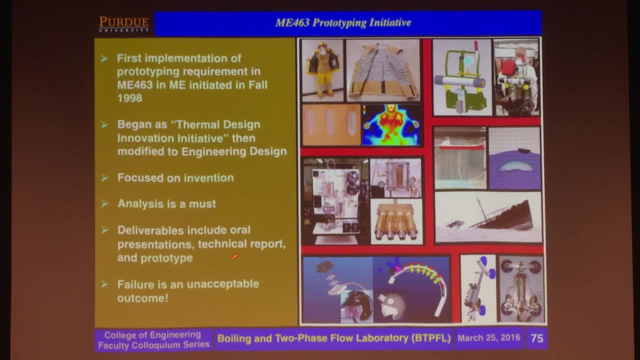 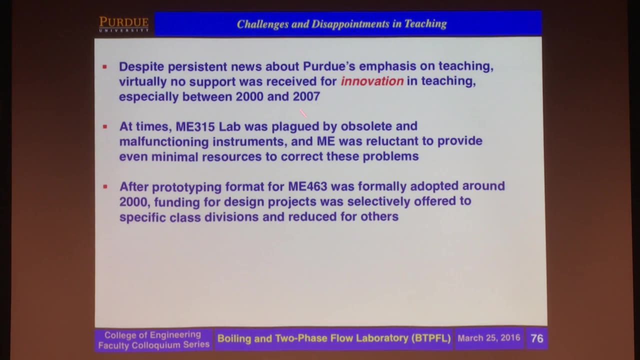 oral presentations, reports and a prototype, And they can't fail. I warned them: if you fail at the end I'm going to get a grade. I lied a little bit. Now here's a point of criticism here, Despite persistent news. 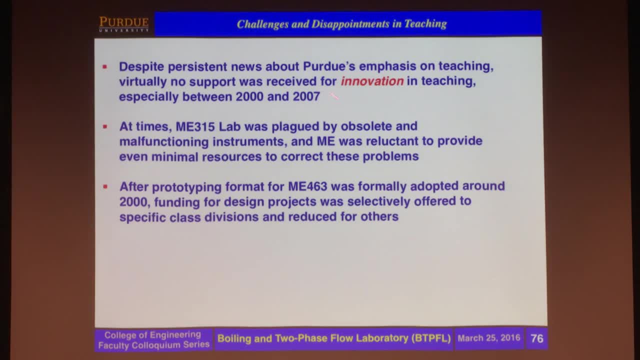 about Purdue's emphasis on teaching. virtually no support was received for innovations in teaching, especially during this period. Now Anil is sitting here. He should be happy because he came after 07.. But this is true. It was an extremely 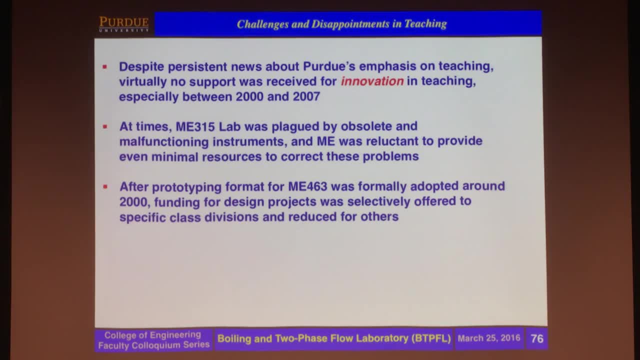 extremely frustrating period And, for example, every 315 lab we passed through a period where voltmeters were failing and we had no resources to repair them Literally- And I would go and argue about differential fees and other things- Never got a penny. 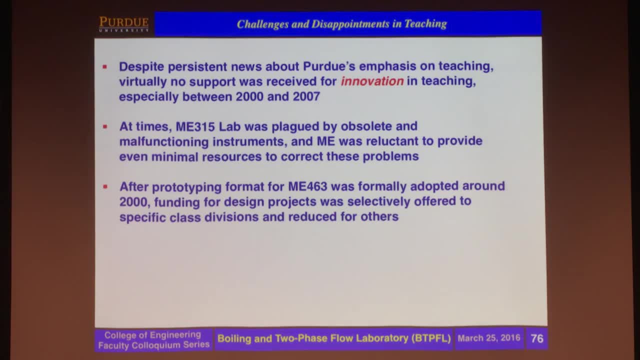 So what I did is I talked to Paul Zmola. He's somebody who donated money to us- And I told him to please dedicate the money that he has in mind that year to ME315 lab, And he gave us $20,000. 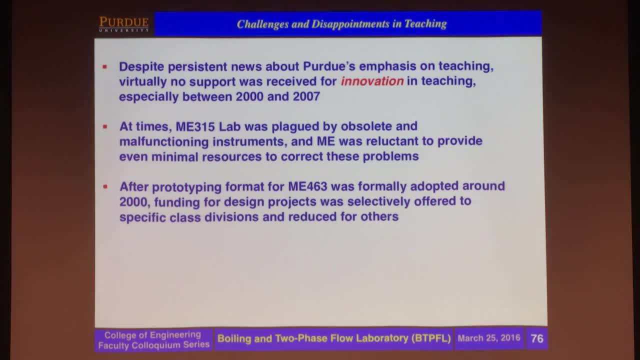 And we lived off that for four years, Literally. And I was surprised that after the prototyping format for senior design was formally adopted, suddenly we didn't receive any funding for it, although everybody was using it. I don't know. And a few thoughts about research. 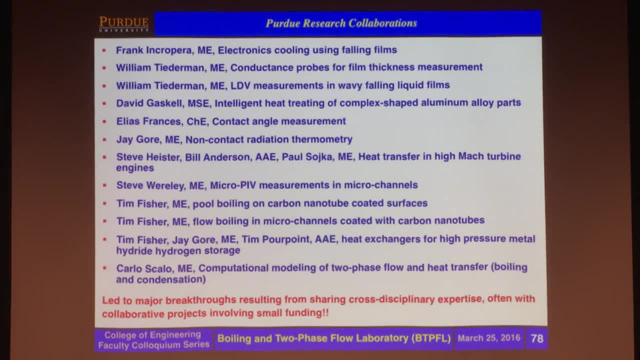 as well. One thing: collaboration, Something I want to mention. I've collaborated with a lot of people over the years And it's absolutely amazing how much you can do with collaborative work. Major breakthroughs are possible. For example, I talk about materials processing. 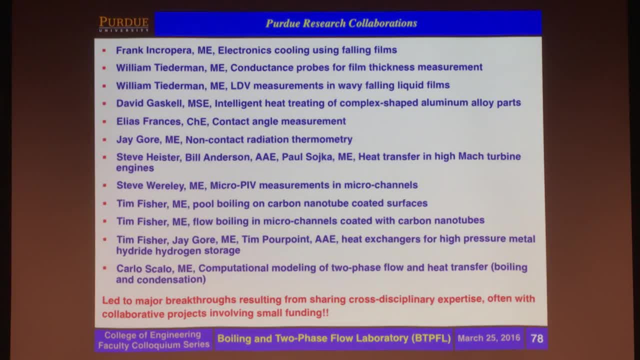 When I started the work. I'm an expert in two-phase flow. I know nothing about metallurgical transformation theory, So I work with a materials professor, Which for him is a very easy topic. Just by combining it, we were able to do incredible things. 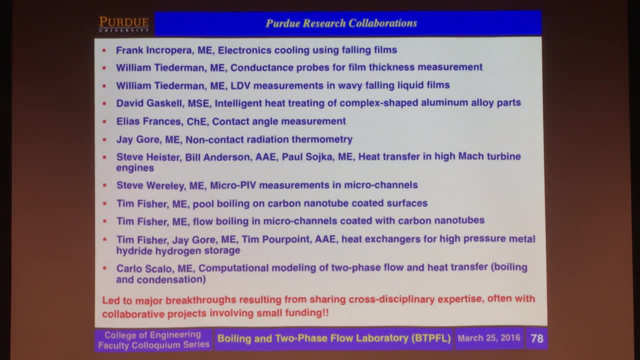 And so virtually every one of these topics led to major breakthroughs Recently. by the way, I got to emphasize Professor Scala. we're delighted about the collaboration Because this is an area where we have very little expertise And he's really providing a lot of assistance. 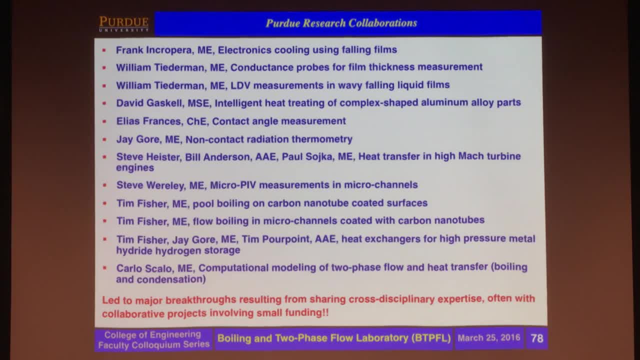 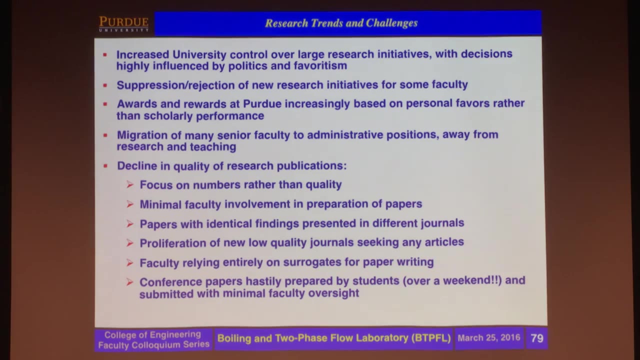 in this area We're collaborating right now. Now, interestingly, these breakthroughs are not money related. In fact, there are some projects here involving a lot of money but relatively minor yield. Okay, Research trends and challenges. Again, this is highly controversial, I think. 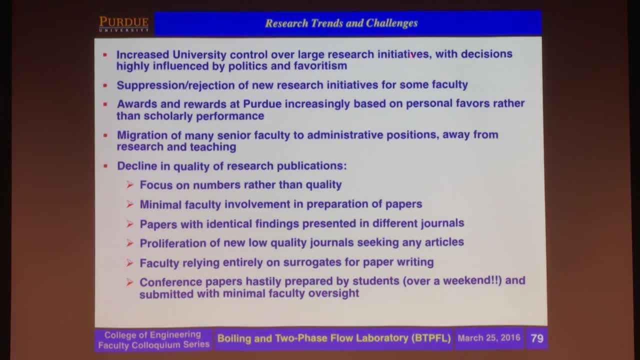 Increased university control over large research initiatives, with decisions Highly influenced by politics And favoritism. Okay, We see a lot of announcements, Big centers, You know whatever. I don't know who's running this, but you feel it's excluding. 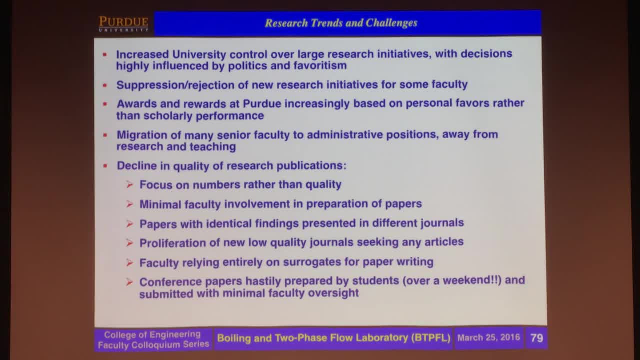 rather than including. in many situations I've seen that firsthand Suppression, rejection of new initiatives for some faculty. I had two enormously large grants in the same year, 2013,, where the attorneys said we're not going to negotiate them. 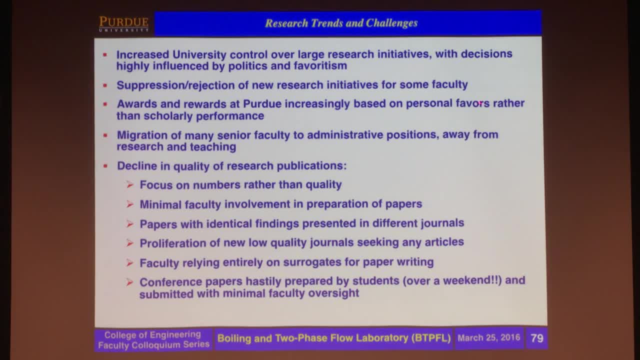 We don't even talk to the companies to try to make them happen. This is at the time when the university was bending over backwards to get other funds. So there is a lot of politics that I still don't understand. Awards and rewards at Purdue. 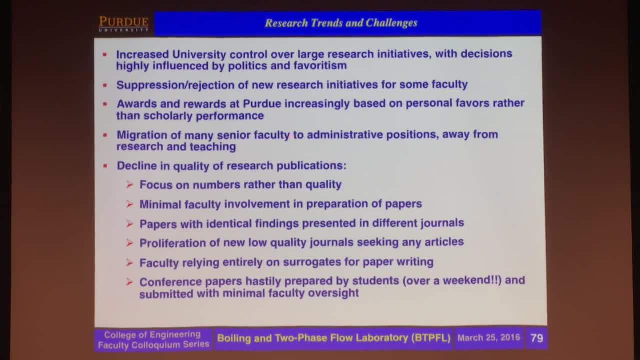 increasingly based on personal favors rather than scholarly performance. It's true This has led to migration of many senior faculty to administrative positions, away from teaching or research. That's a fact as well. I'm not talking about everybody, but I'm talking. 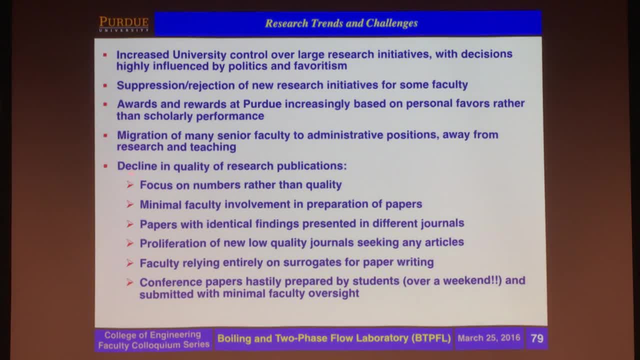 there are certain factors leading to this. There's also something I'm very concerned about, which is a decline in the quality of research publications, With the focus on numbers rather than quality in many cases- I'm seeing it more and more- Minimal faculty involvement. 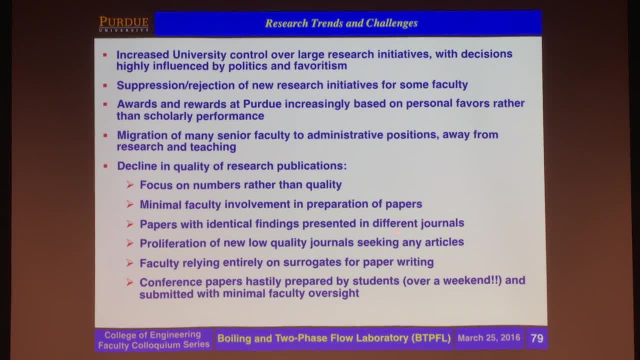 in preparation of papers. I hear it from students as a matter of fact. Well, my advisor doesn't like to spend too much time looking at my papers before we send them Papers with identical findings presented in different journals. Proliferation of new. 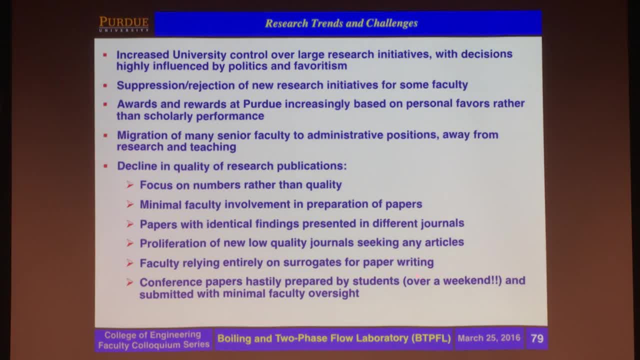 low-quality journals seeking any articles. begging you for articles. I receive those every single day right now: announcements: Oh, we saw your article entitled whatever. Can you write another one without review? We're not going to review it for you, Just send it to us for our journal. 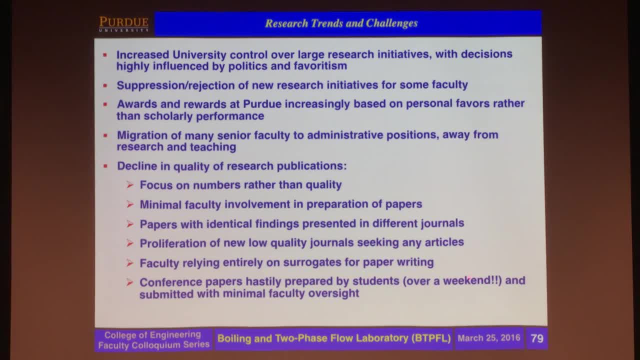 And also some relying on surrogates to write papers. The worst- this is something I had to deal with personally- conference papers hastily prepared by students over a weekend, literally with no faculty oversight. I discovered that when I was working on a project. 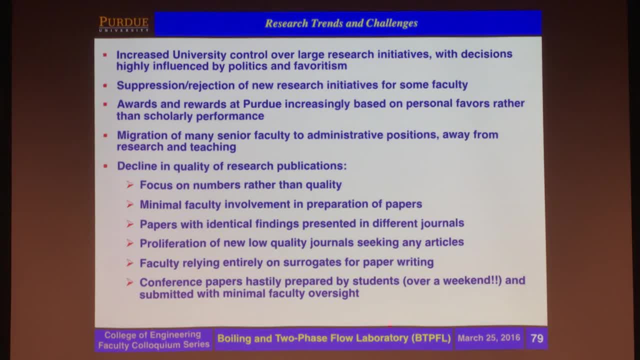 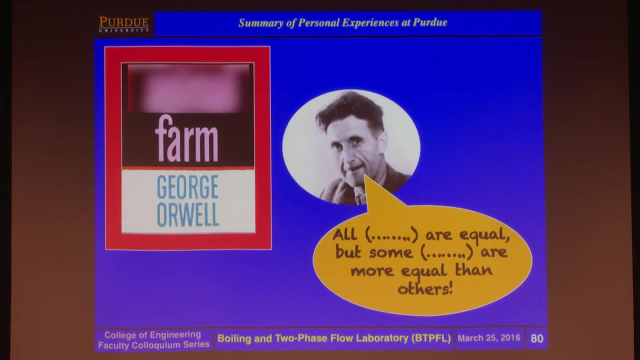 and I asked the faculty member to remove my name from any paper submitted to a conference from that project. I didn't care and I don't want to see my name attached to it, But it's a quality issue And my wife got angry at me for doing this. 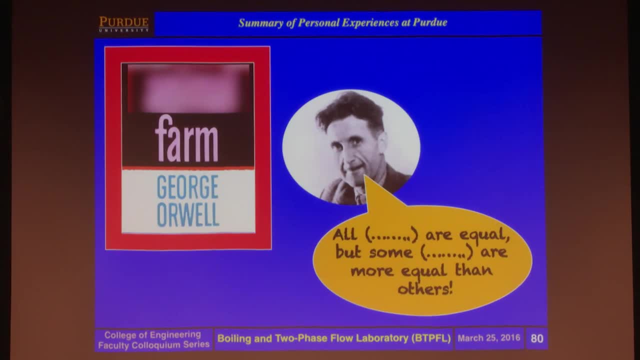 This is the last slide- My favorite author- I don't know if you know his- George Orwell And all whatever are equal, but some are more equal than others. I'm hoping when I retire I forget that this happened, but that's the way I felt. 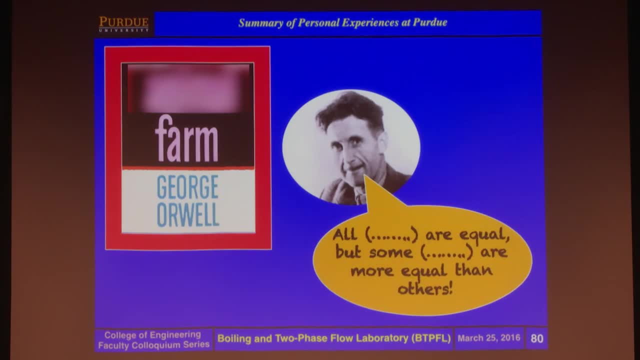 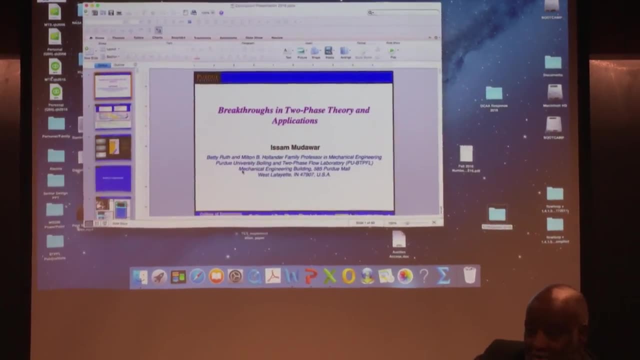 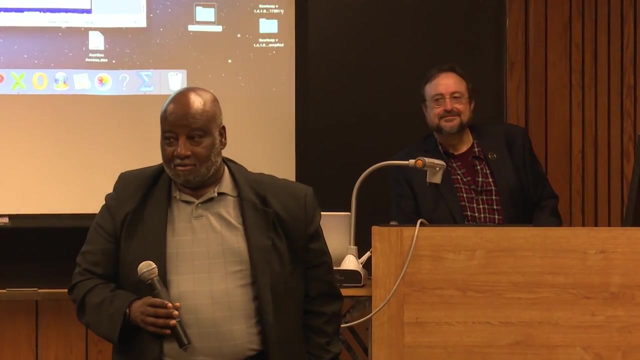 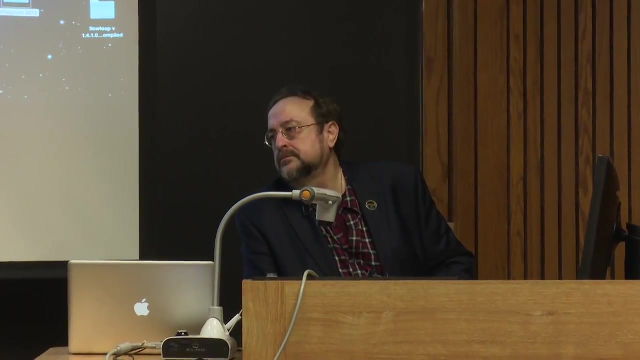 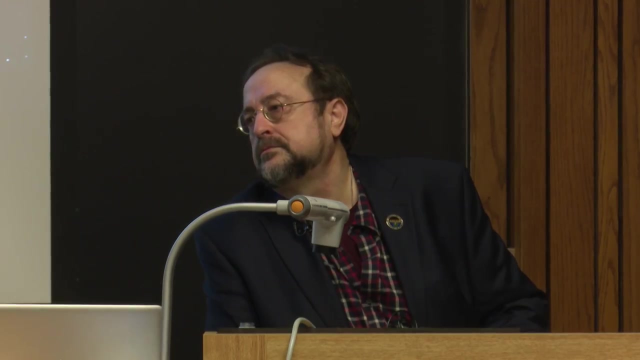 Thank you. We will open the floor for questions. Yes, You mentioned several fluids, such as water and R134, also JP8, and then you mentioned the importance of the critical point. Yes, Now, if you go past the critical point, pressure-wise. 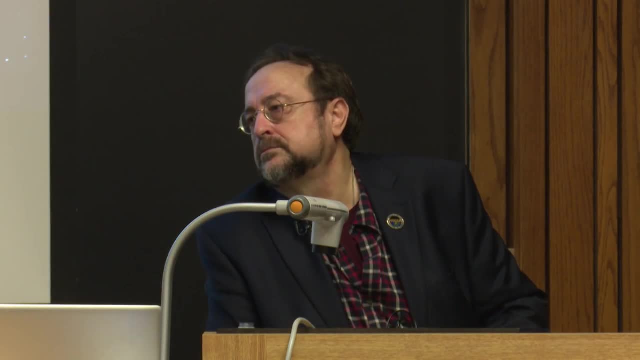 so you go supercritical P, then you don't have a proper boiling, you have a pseudo-boiling, So there's no interface. Is that better for CHF, or is that something you guys, people in this community, avoid? Is it a structural problem for the heat exchangers? 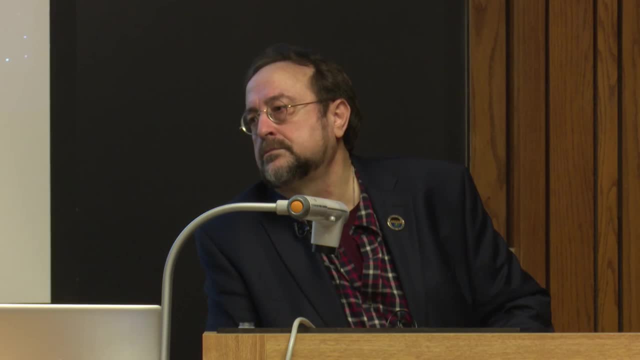 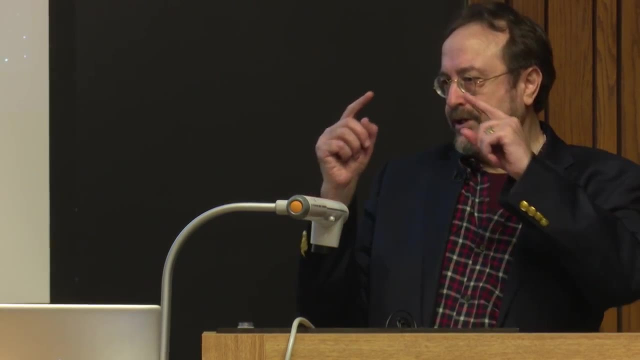 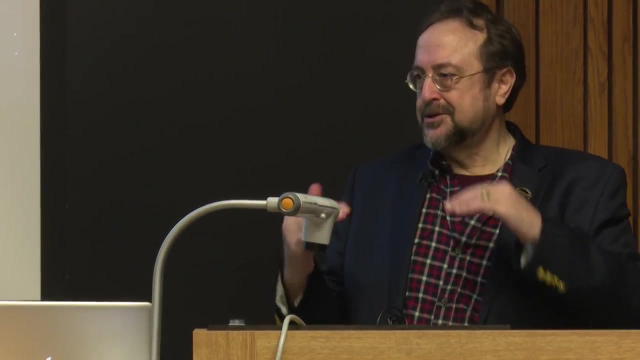 to be designed at those pressures? Are those conditions that are probably worse for what you're trying to achieve, or are they better? Any time you get close to the critical point, your CHF, for all practical purposes, is zero anyways. So as you're going up in pressure, it actually peaks. for example, for water it peaks around 50 bars. It's low at one. atmosphere peaks around 50 bars. Then when you hit the critical point, it's practically zero. So you are talking about the range nobody's interested in. 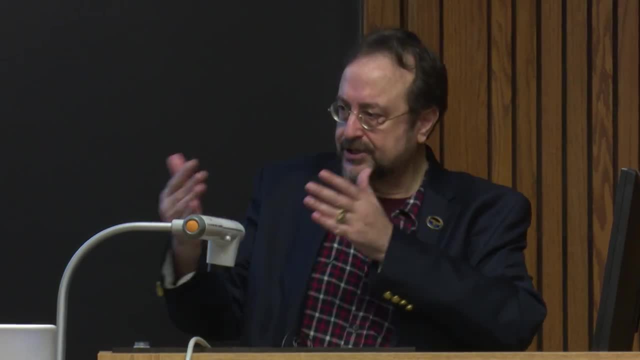 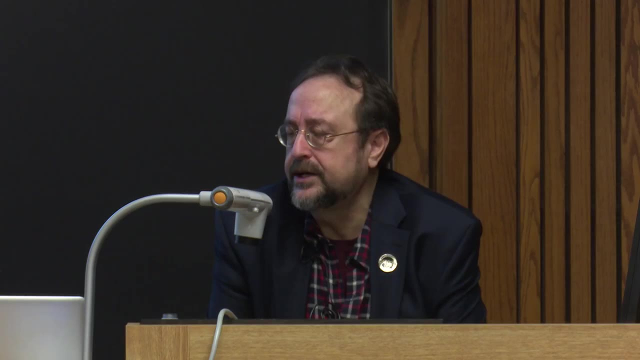 If you look at the nuclear reactors, for example, you got 50 bars, 70 bar, because they want to take advantage of that sweet spot. And if you go on the other side, if you go super critical, There is no indication. 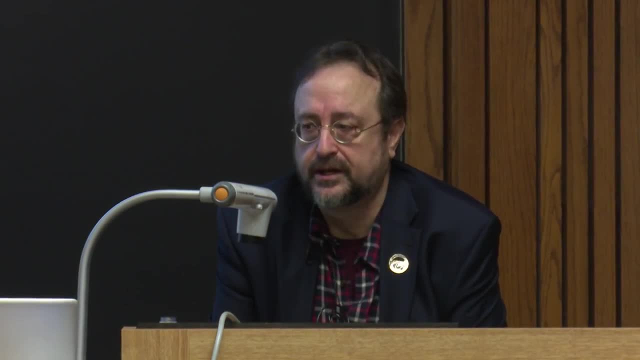 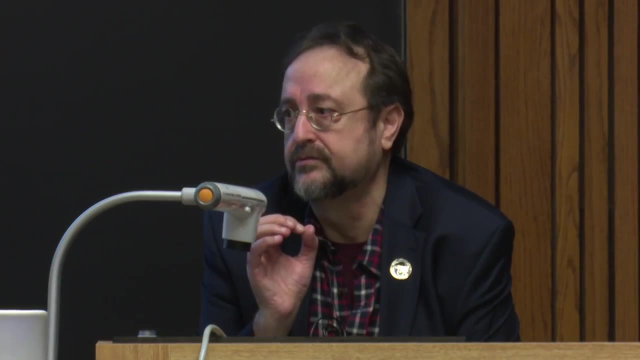 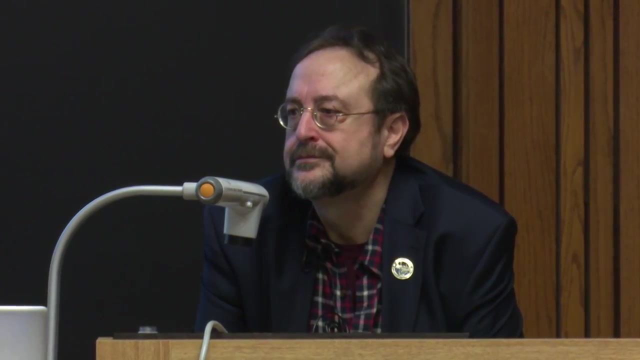 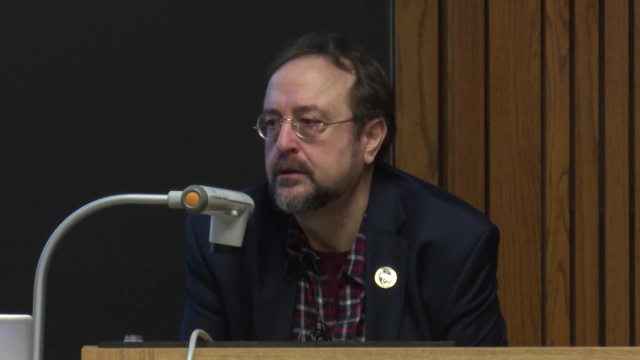 that it is really advantageous from a critical heat flux standpoint. Having said that, not many people have done work in that area. that is really conclusive. Yeah, what is the state of theory? for you know, you showed boiling starting all at walls, And you know. 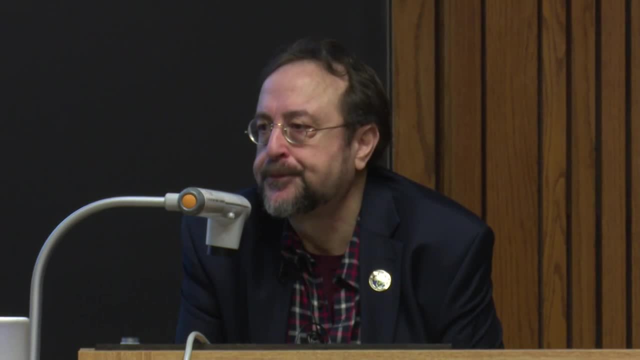 if you have a homogeneous fluid that's above the boiling temperature, is there a theory for formation of bubbles in that? Or you know, if you have a fluid where you have bubbles and the fluid temperature is below the condensation temperature, how long it takes? 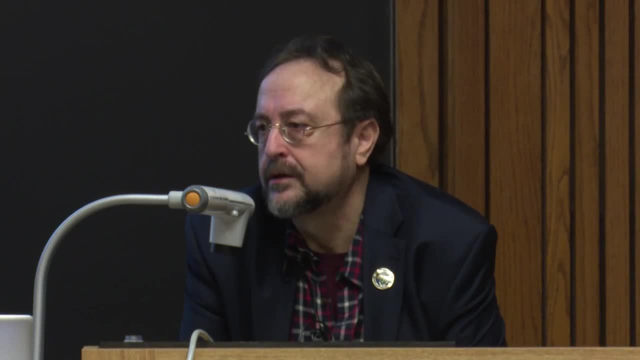 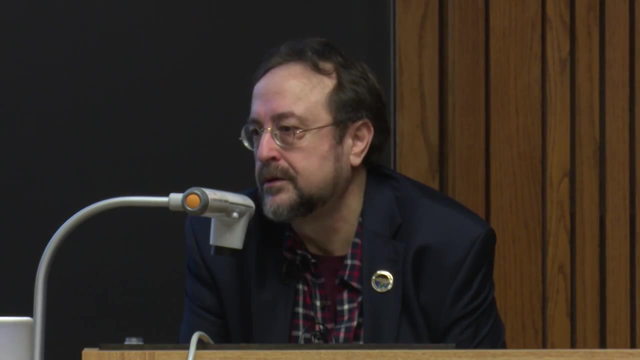 those bubbles to collapse. Of course there is a lot of work about that. I mean you know there is a lot of work about that. I mean you know there is a lot of work about that. I mean there is a lot of work. 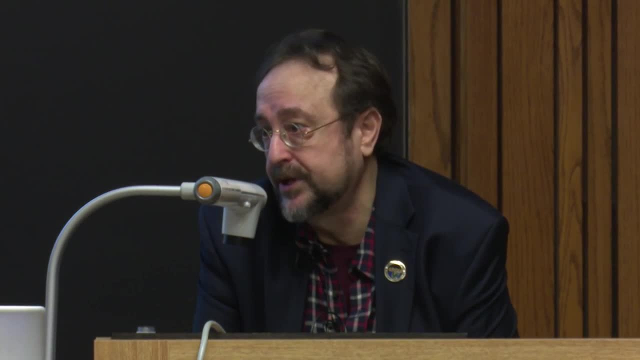 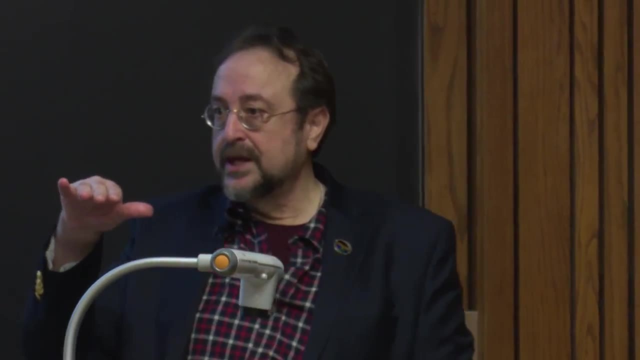 about that. I mean, you know there is a lot of work about related to bubble dynamics. It's all under the title of bubble growth theory And it gives you diameters as a function of time. There is, there are two regimes. 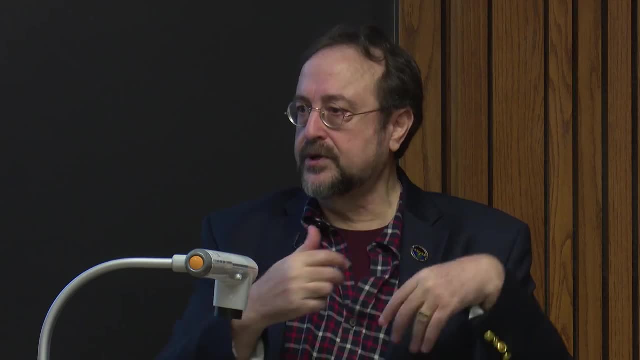 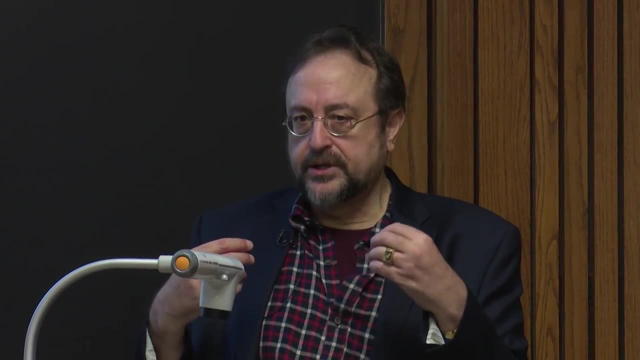 actually well identified. One of them is a dynamic regime, Another one is a thermal regime, okay, which is much slower, But the theory has been around for a while and there are publications in those areas available. Is that all connected with the 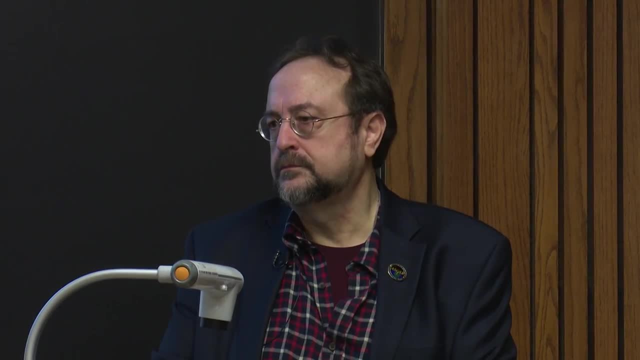 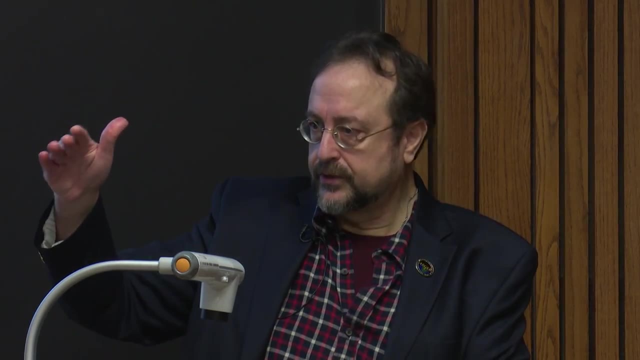 you know, like the theory of metastable equilibrium in these fluids also. No, That's. that's a totally different topic. Okay, what I'm talking about is the dynamics of bubble growth under low pressures versus high pressure. You may be talking: 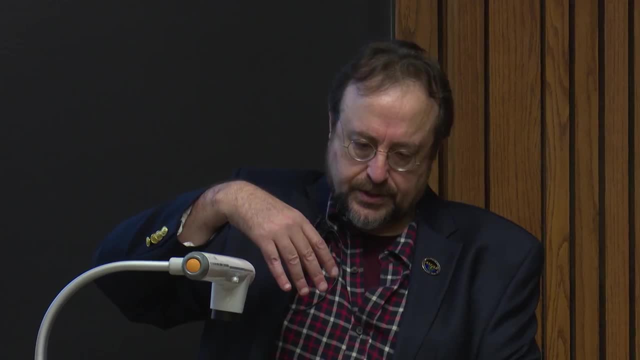 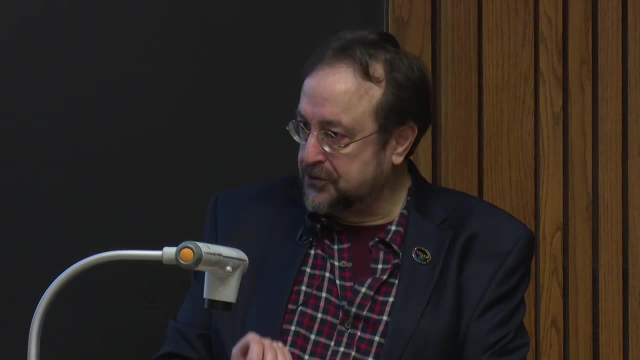 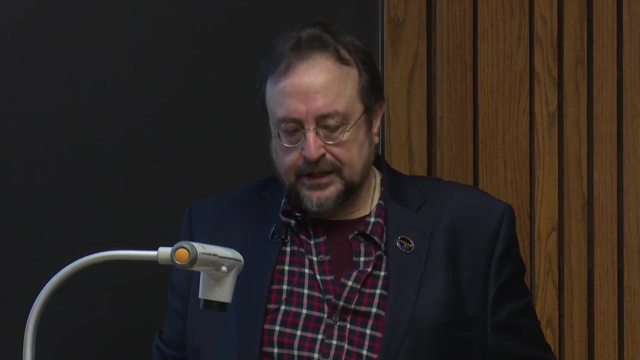 about situations where you have, like a mirror surface, mirror polished surface that doesn't promote boiling, yet you do finally end up with bubbles forming on the surface. So you know that's that's a very interesting topic. Okay, that is. 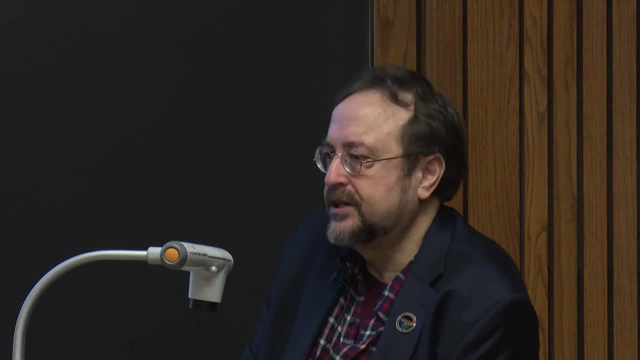 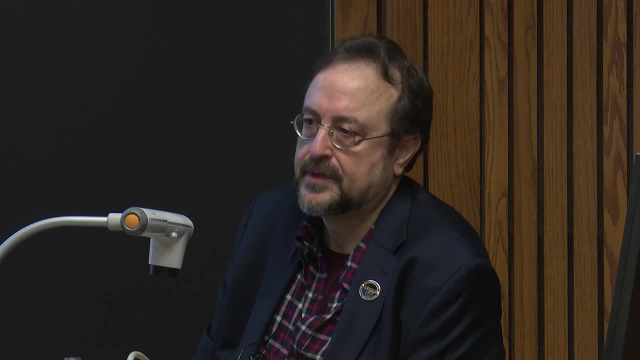 superheated liquids and subcooled gases. Absolutely They. that's usually addressed from a thermodynamic standpoint rather than mechanistic heat transfer standpoint. A lot of the work that you see out there, But it has been addressed and, and you see it a lot. 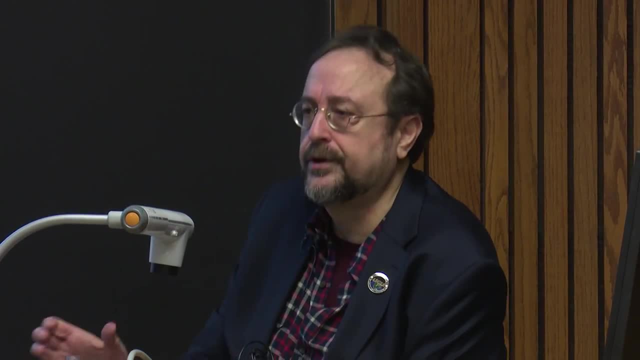 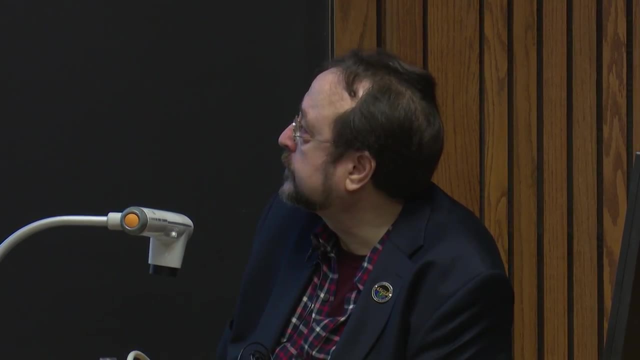 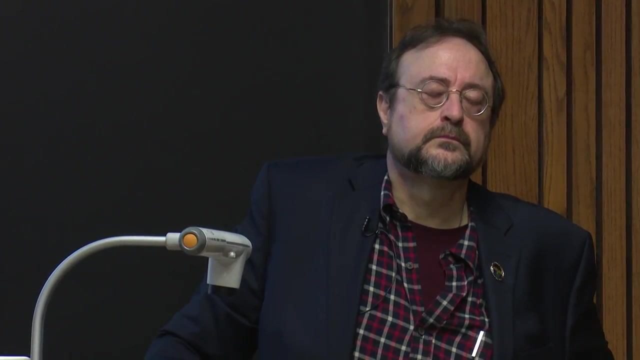 in chemical engineering, as a matter of fact, more than you see it here in mechanical engineering. So, Issam, so after 32 years of research and teaching, so where do you want to go from here and where do you want to be in 10,? 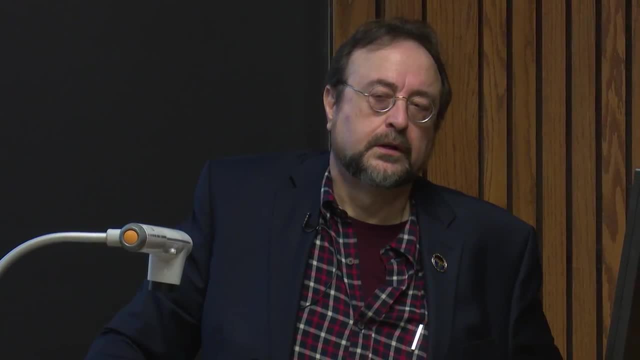 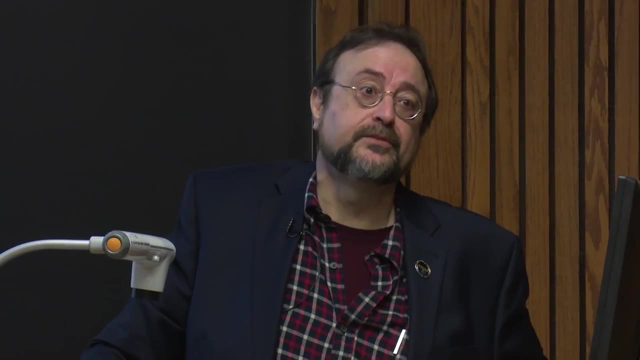 20 years from now, scientifically and technically. Well, I'm going to age here because I love research. I think research is extremely exciting and actually, as I'm aging, I'm finding it more and more exciting. Believe it or not, I'm constantly. 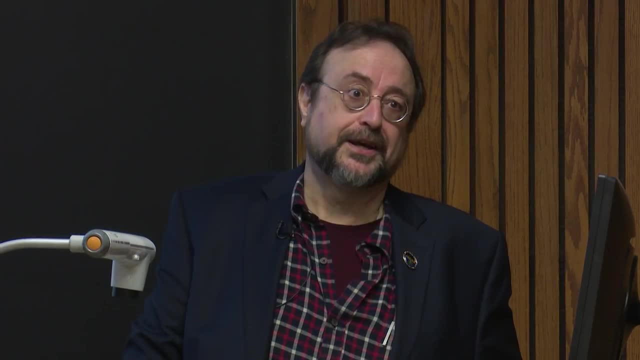 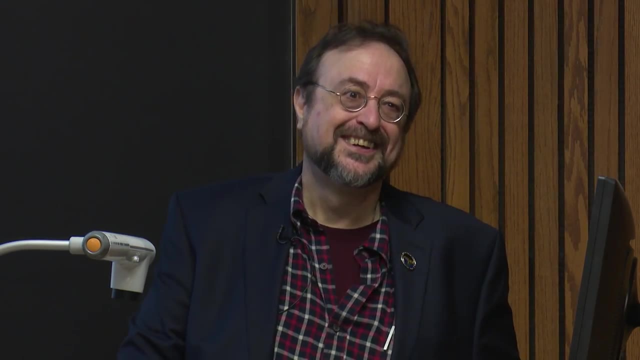 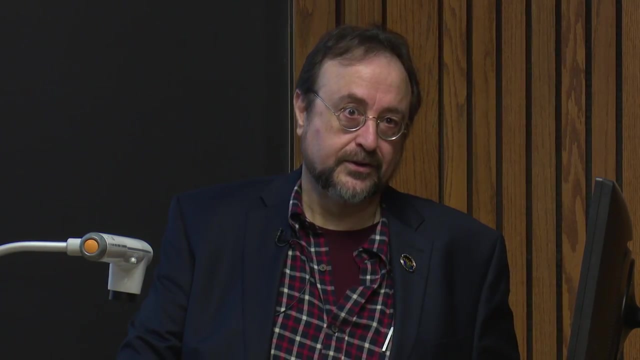 asked to think about, and I'm constantly asked to move somewhere else and serve in an administrative capacity, and I'm consistently saying no because I don't see myself doing that kind of work at all. Okay, and the fact that I'm doing my research, along with the work. 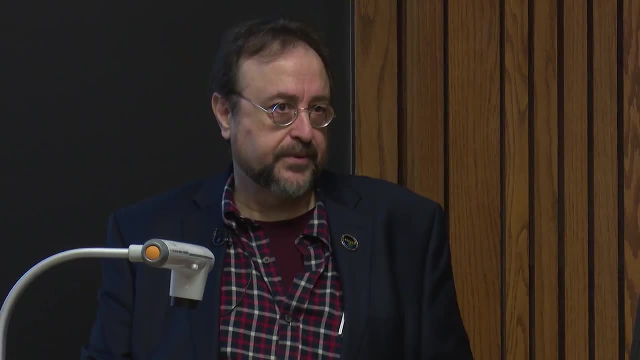 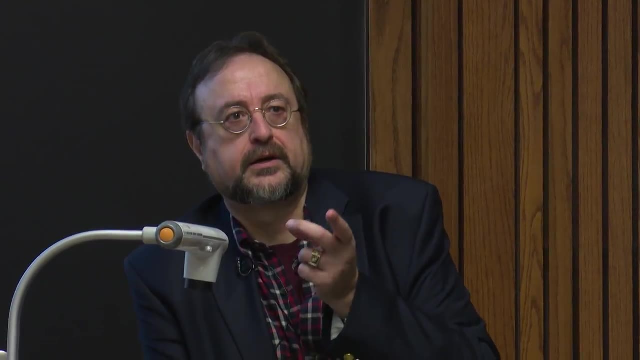 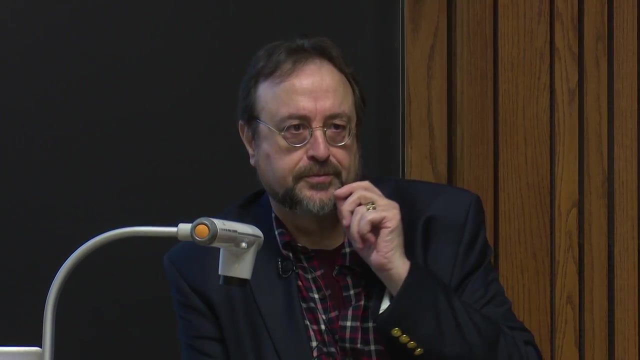 I do in my company, which complements the things that I like to do. I'm very happy with that, You know. let me tell this to you: Recently it was at a NASA event. There's a gentleman who is a fellow in a famous 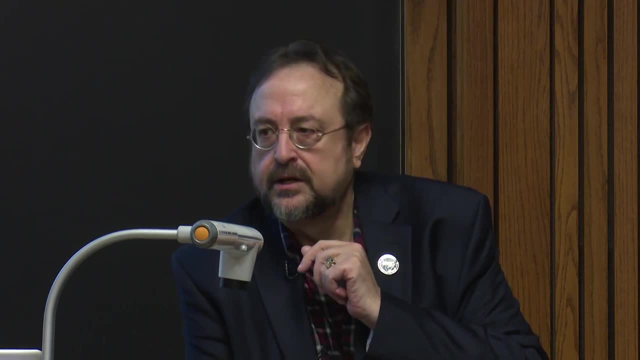 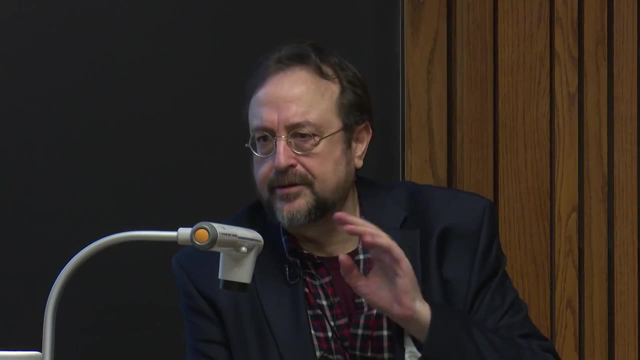 aerospace corporation- I don't want to mention his name for a particular reason- Well known for his patents, inventions in aerospace, He's a consultant for NASA forever. You know, anytime they have a review event for NASA related activities, they bring him on board. 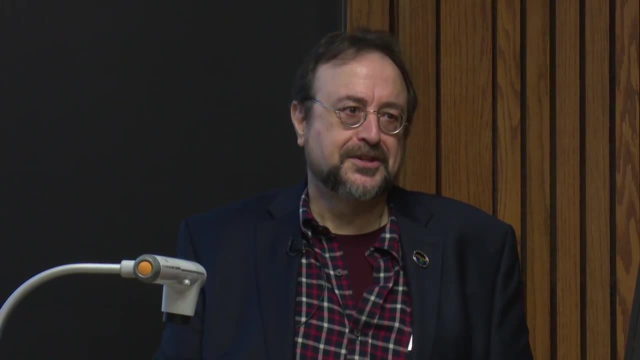 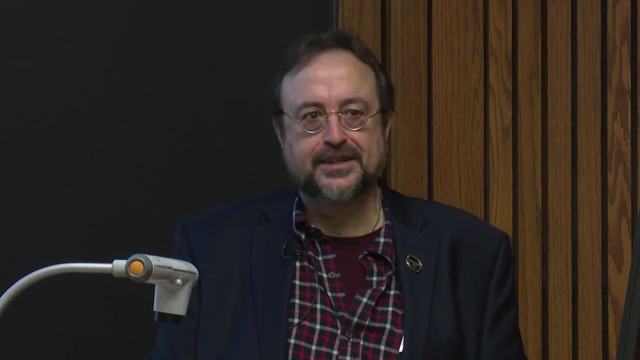 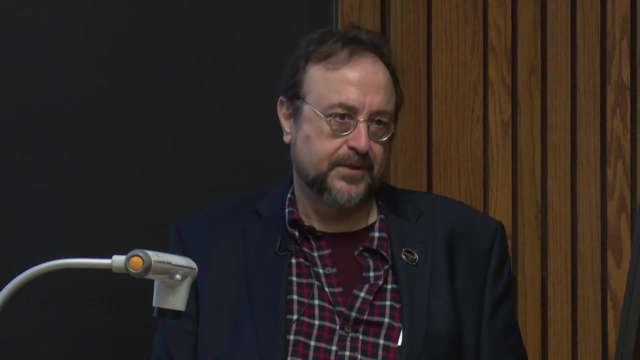 and he just retired. So I asked him what he wants to do. He wants to become a professor. He said I'm not going to sit home and my company doesn't allow me to continue at the age that I'm at. So 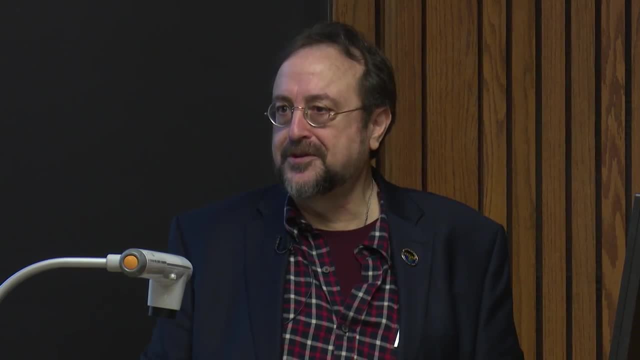 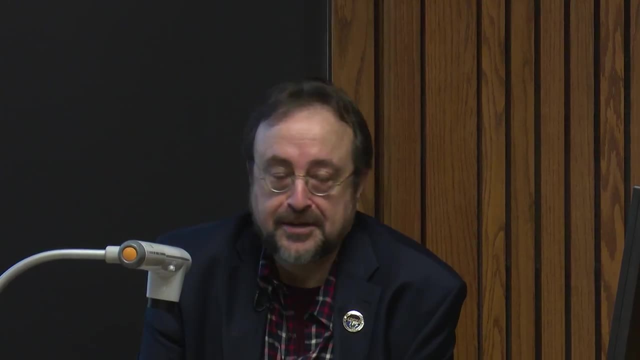 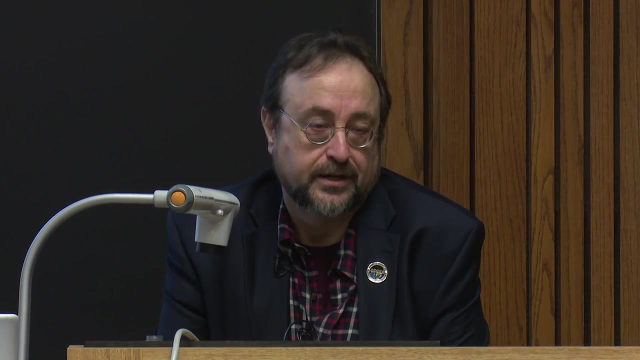 he literally found a university that wanted to capitalize on his skills and he's going to be a university professor until he hits whatever age you know- 85,, 90. And he's extremely delighted with his career. Okay, unfortunately it's plagued. 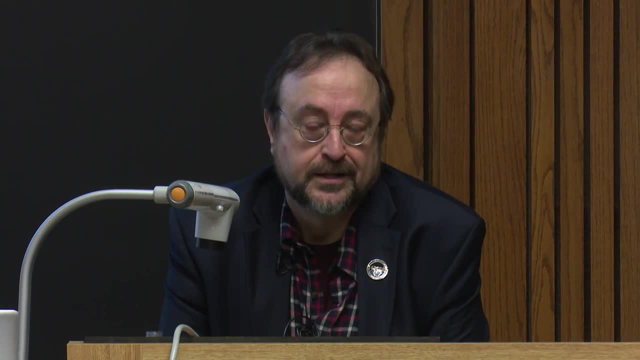 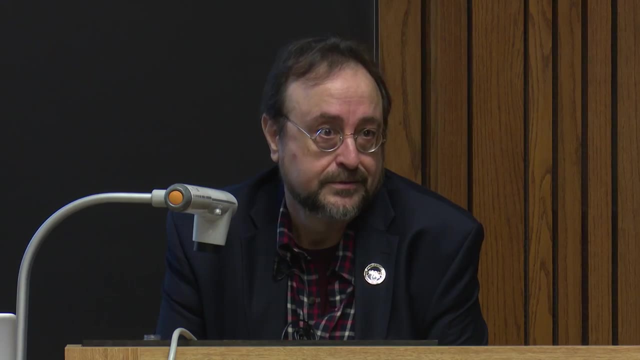 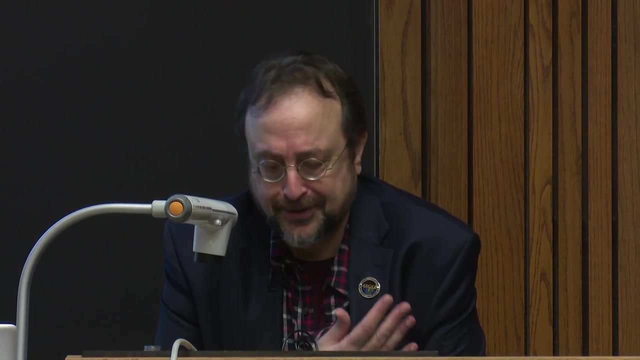 by politics, but these things come and go with time. So the short answer: I really enjoy my teaching and I love my research and I love the work that I do at the research park. The only thing I don't have time for is my hobbies. 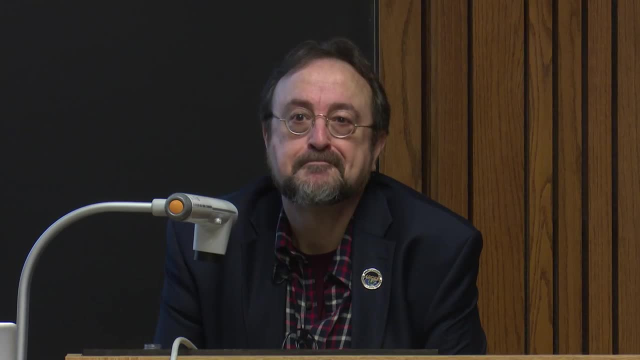 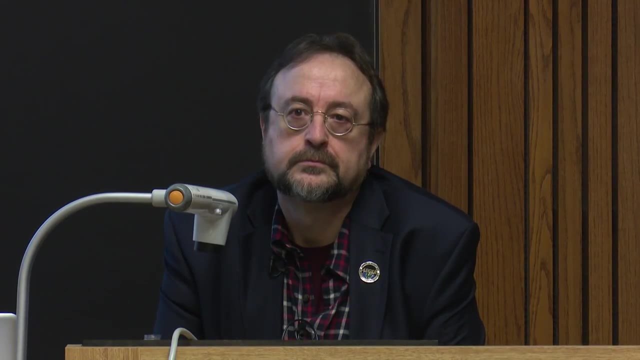 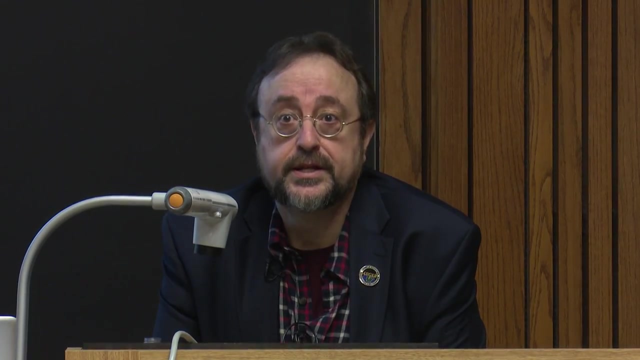 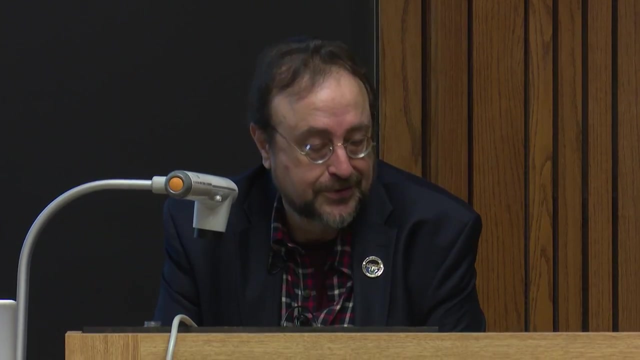 I would rather do some oil painting, but I don't have time for that, So I'm going to do some other work. Okay, so you have a lot of work you were doing, and the heat transfer doing during that process Is there. 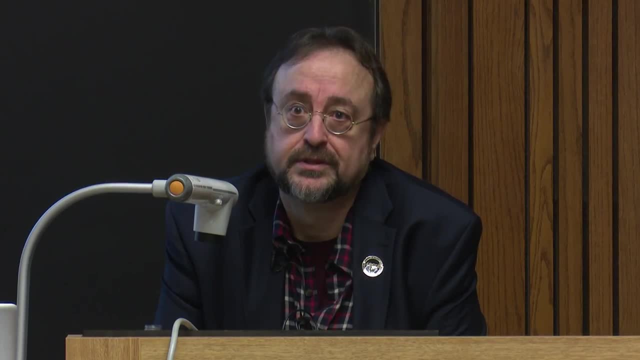 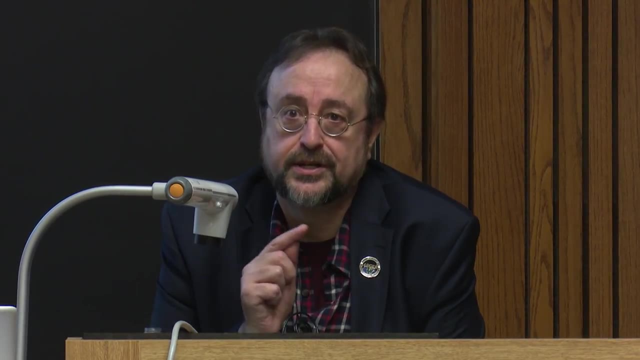 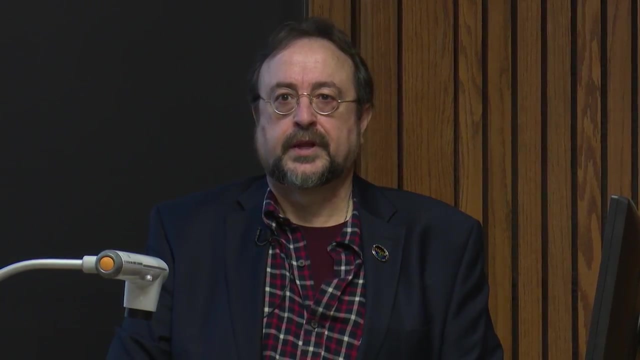 a significant expansion of the metal as the hydride is formed. You absolutely have to account for that and you have to account for some reduction in the performance of the heat exchanger. You can't fill it as much as you think you can because of 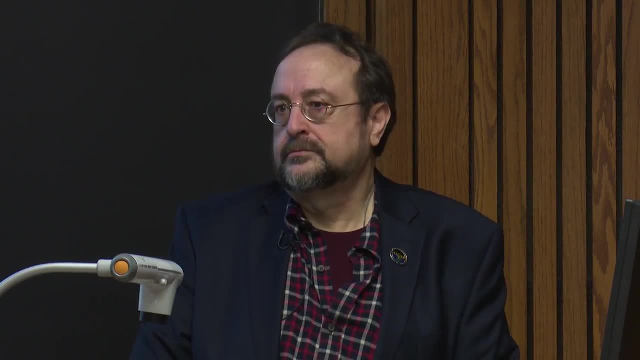 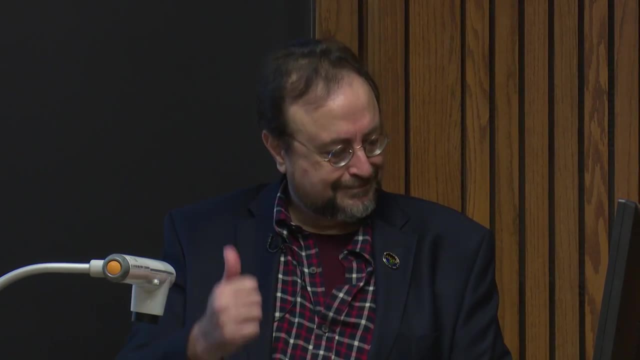 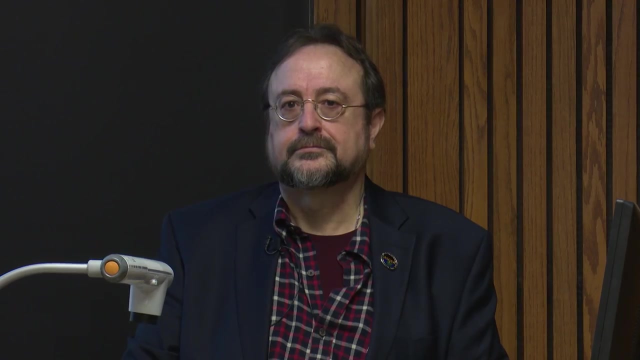 that factor. Well, once again, if there are no further questions, I want to thank you for an excellent presentation. I was quite fascinated with all of the things that you're doing and all of the innovations. Please contact my office, because I would. 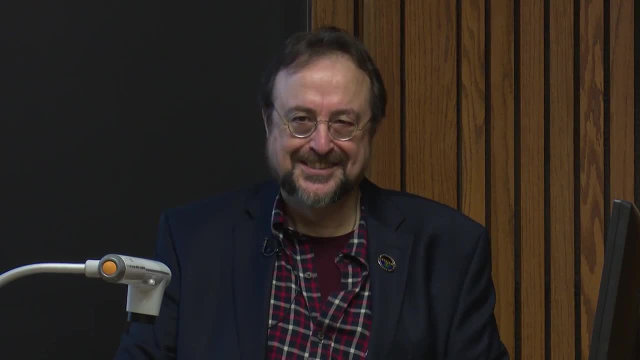 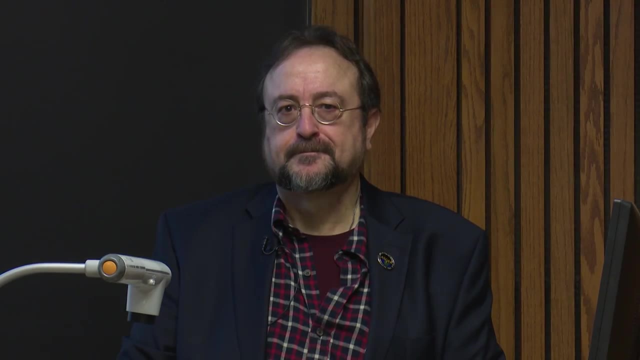 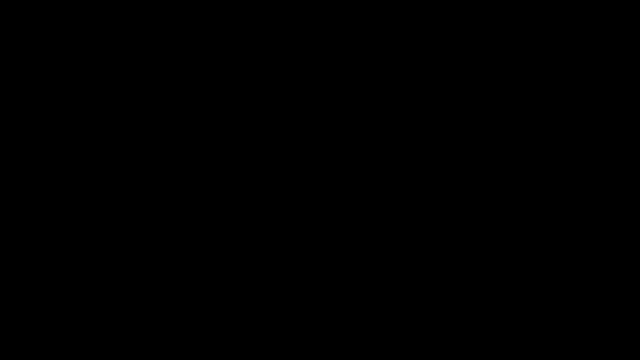 love to. Well, we're building one right now, actually, and when it's done I'll probably show it to you. Okay, well, thank you, Thank you. Give him a hand one more time. Thank you very much.